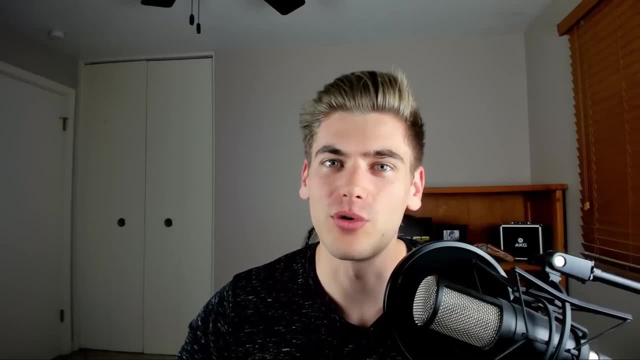 fit into this video, but I do have an entire full course on React that covers all of those advanced topics I can't in this video, and it also covers the mindset shift and the ability to think in components and write efficient React code. So if you're interested in checking that out, make sure. 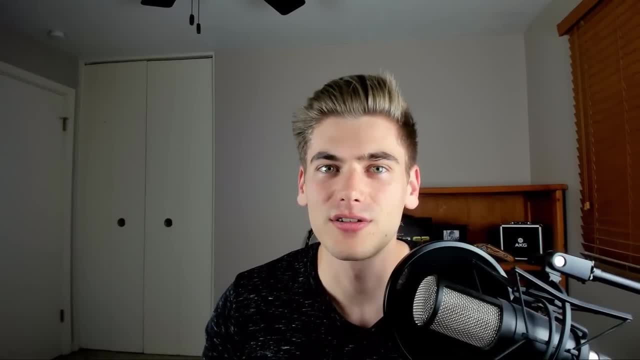 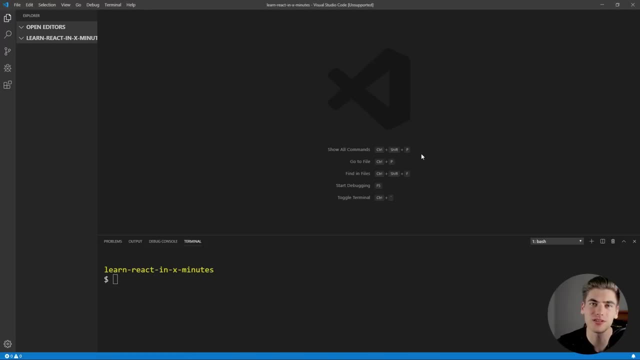 to click the link in the description below in order to buy that course. So with that out of the way, let's jump into this tutorial. To get started, I have Visual Studio Code open to a completely blank project, And the first thing we need to do is actually create our React. 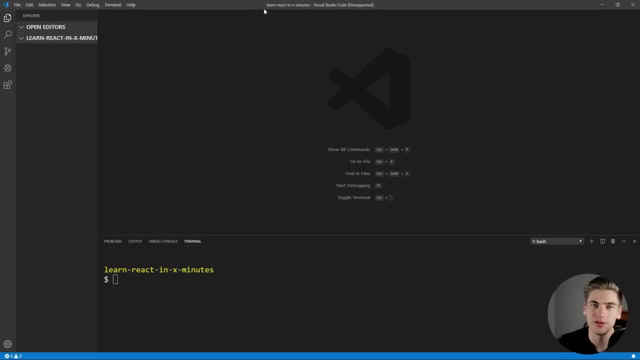 application, And to do that you need to be inside of a folder that has no capital letters and no spaces in the name. Our folder is called learn react in x minutes, with dashes in the name instead of spaces. So this is going to work for us just fine, And what we need to do is we need to make 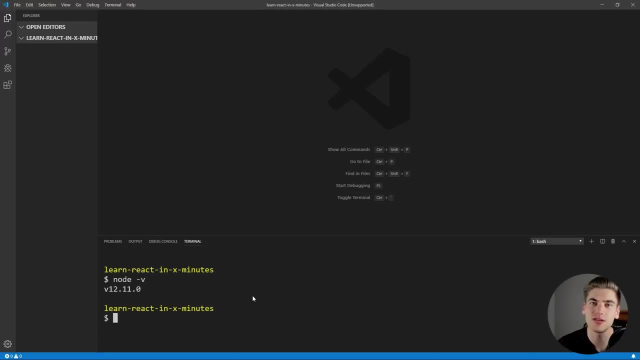 sure we have node installed by just typing node dash V, And if you see a version, then that means you have node installed. If you don't see any version or you see an error, that means you do not have a version. So if you don't see a version, then that means you have a version, And if you 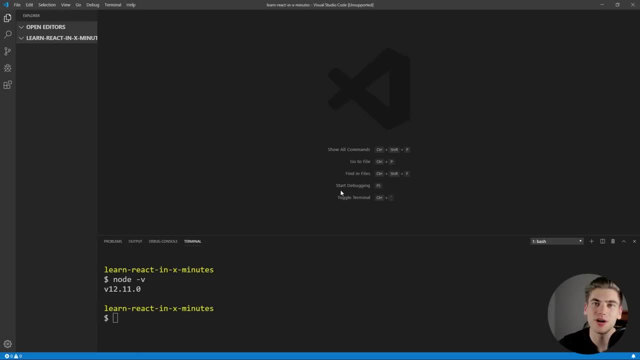 have node installed and I have a video on how to install node linked up in the cards in the description below, So you can check that out in order to figure out how to download node. Now, once we have node downloaded, we need to run is npx, which is a lot like npm, But instead of downloading. 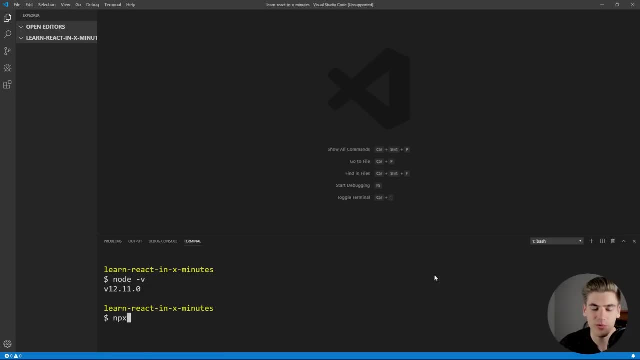 something. it is actually going to run that command for you And we want to run the command create react app with a period at the end. essentially, that period says: use the folder we're already in to create the application inside of, And when we hit enter, 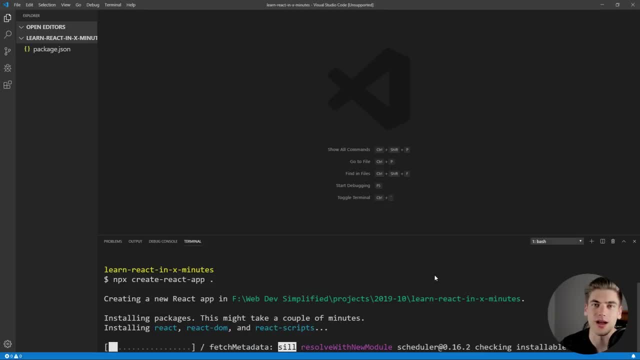 what this is going to do is it's going to start up and create our entire react application. It takes quite a while to download everything, So I'm going to come back to you when it's finished downloading. So now that that's finished downloading everything, you can see that you have a ton of new. 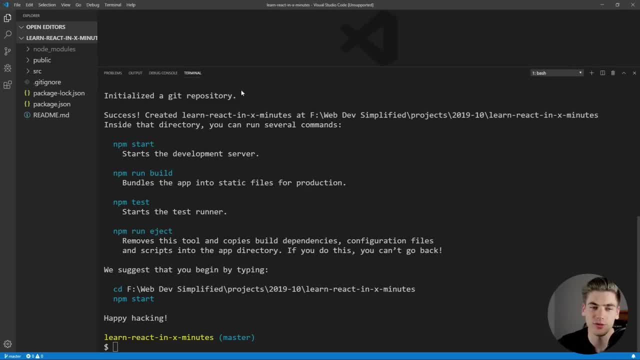 files and folders on the left hand side here, And if we scroll up our terminal, you'll see that we have a bunch of commands we can use inside of our application, And the main ones you want to worry about is npm start, which is going to allow us to start up our development environment, And then npm. 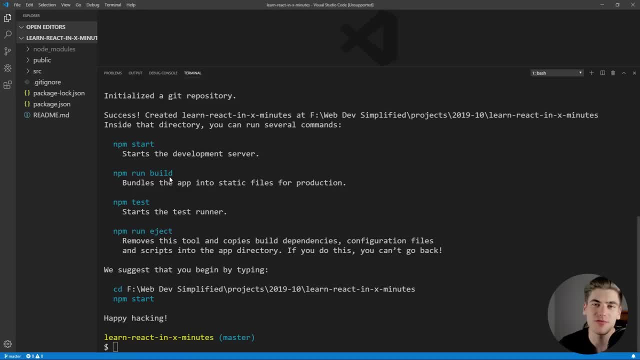 run build. this is going to build our application inside of our application. So we're going to build our application, minify all of our files and give us a production version of our application that we can deploy to a server somewhere and actually access on the internet. So npm, start for. 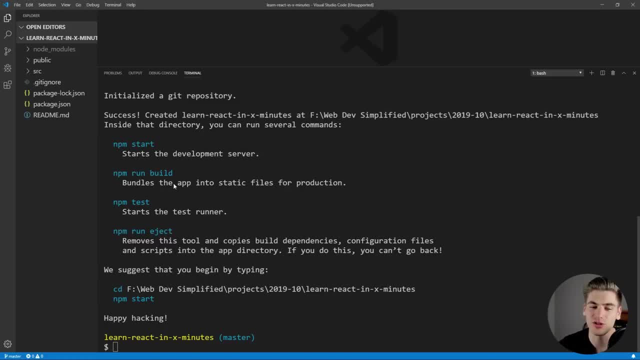 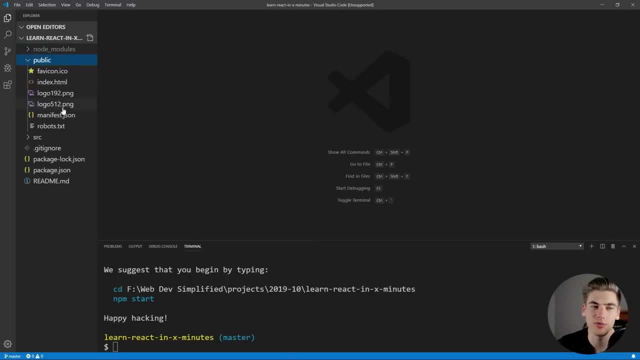 development: npm run, build for production. That's essentially all you need to know. Also, we can take a look over at the files that we have over here. node modules is all of our libraries and our public folder. we have essentially our HTML file, And what's special about this HTML file? is it only? 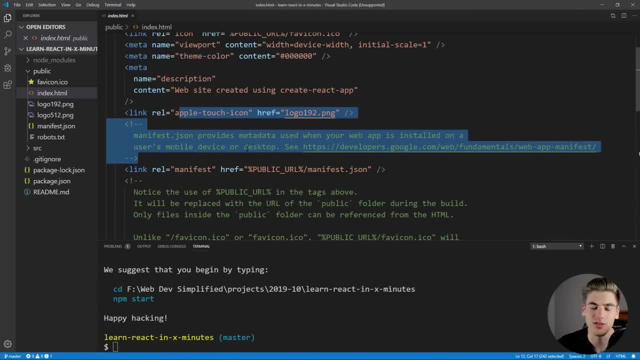 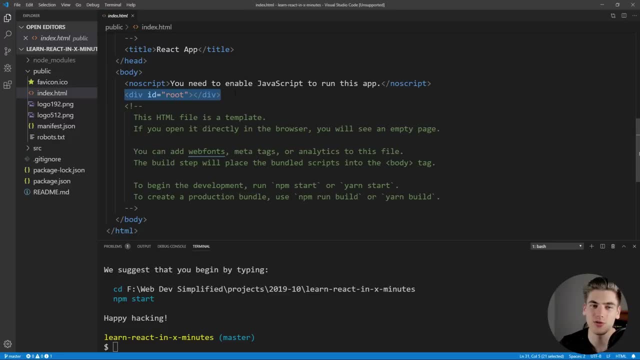 has one div, which is our root. there's no stopper, And then we have the file that we're going to use for the style sheets. there's no script tags. nothing is inside of here except for this single div, which is route, And all of our application is going to be put inside of that route. div React is. 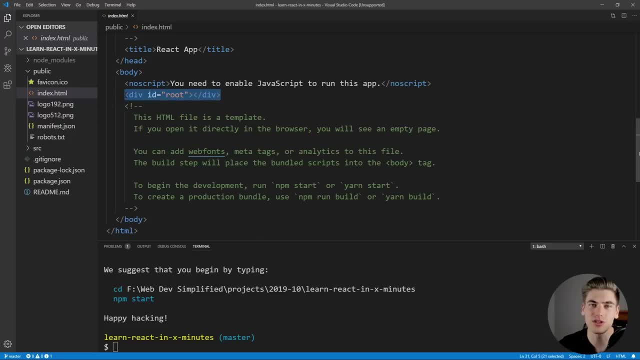 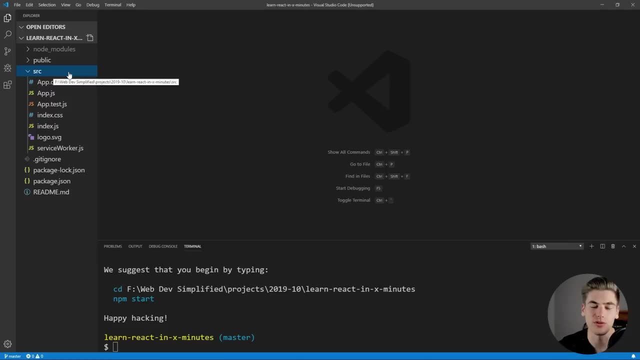 going to generate our HTML and put it inside of this div here, So our HTML is very basic for this application. Really, the main meat and potatoes of the app is in the source folder, where we have all of our style sheets, JavaScript, test files, logos- literally everything in your application, that is. 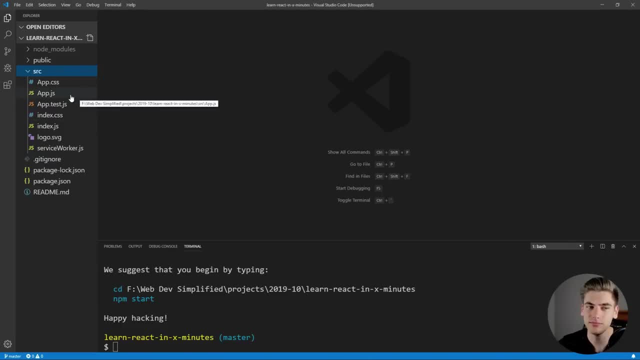 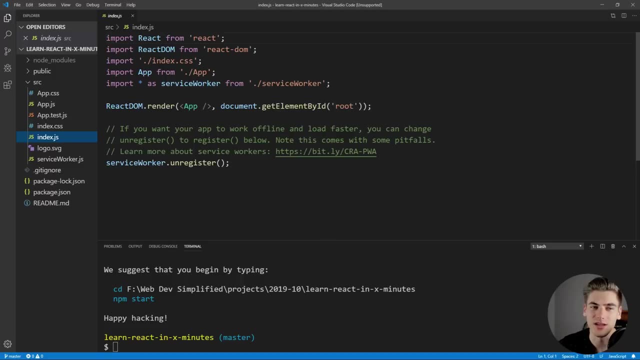 part of your source files, of this source folder, and the main ones i want to look at is our indexjs, which is where our application starts, and what this is doing is it's saying react, dom, render, which is saying render the content we pass in here at a certain element. so you can see we're getting the root element, which 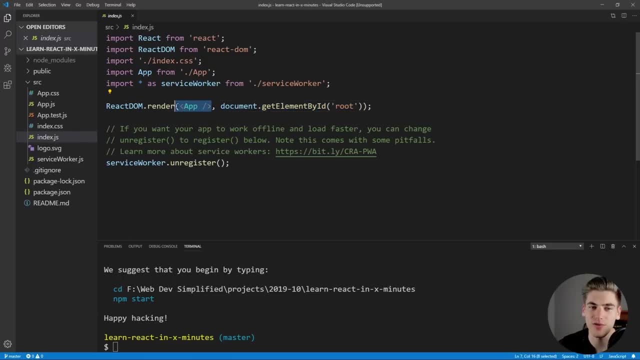 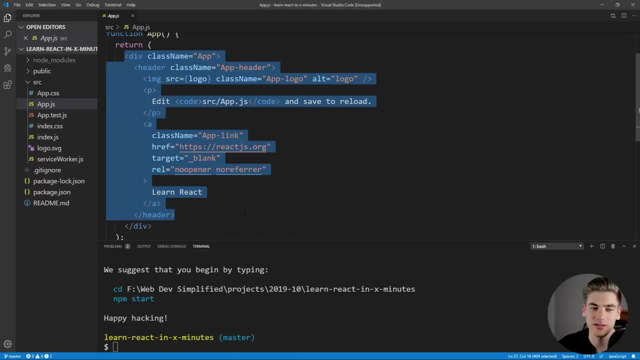 is that element inside of our html and we're rendering everything inside of our app component, inside of that root element, and if we go into our app component, you can see it's rendering just this basic boilerplate code that comes when you create a react application. so let's actually 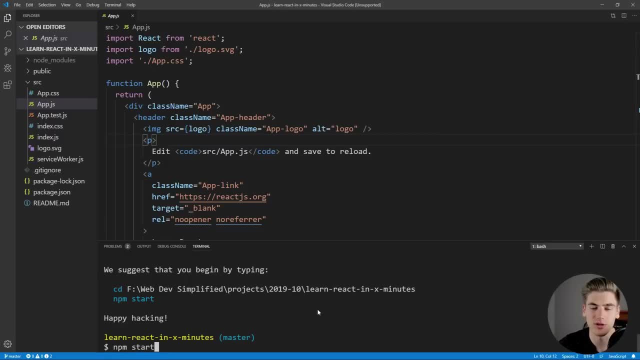 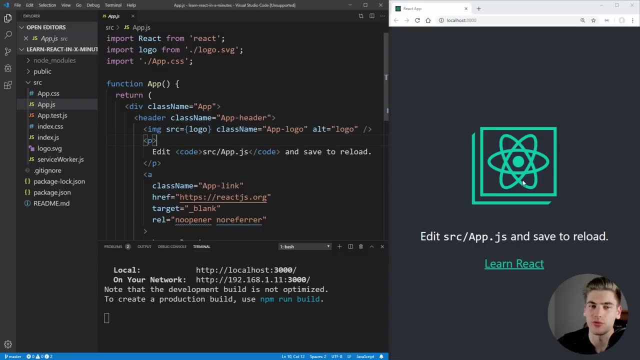 start up our application by running npm, start to see what it looks like, and this takes a little bit, but it's going to open up on our browser for us. now, with that loaded up, you can see our application over on the right hand side and if we change something, for example, if we change this: 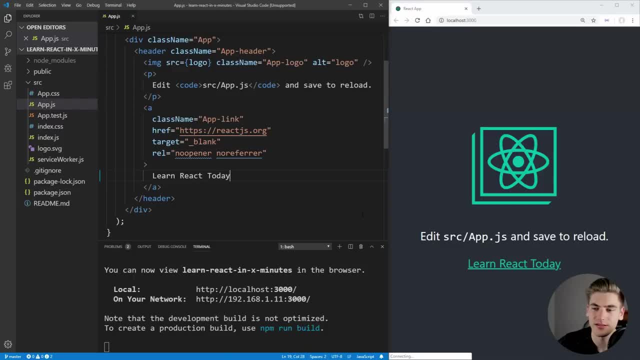 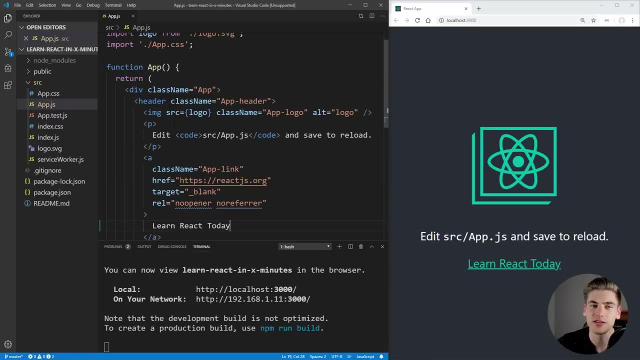 instead of saying learn react, we say learn react today and save. it's going to automatically refresh over here for us, which is a really great aspect of react. but for our use case we want to actually remove all this boilerplate code, so we're just going to return null here. 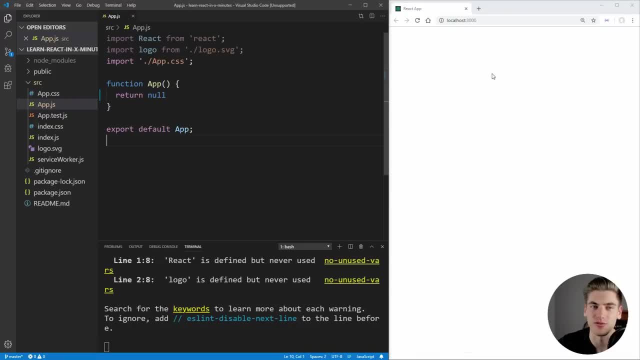 and if we save this, you should see, now nothing is showing up on the site over here also, we can remove this extra code for the css and logo import, as well as removing this test file, all of these css files, the logo file and also inside of here. we no longer need this service. 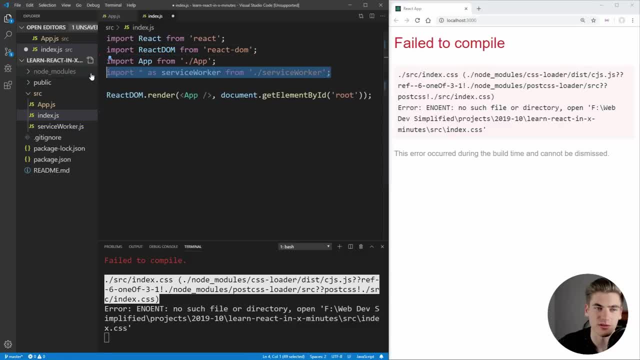 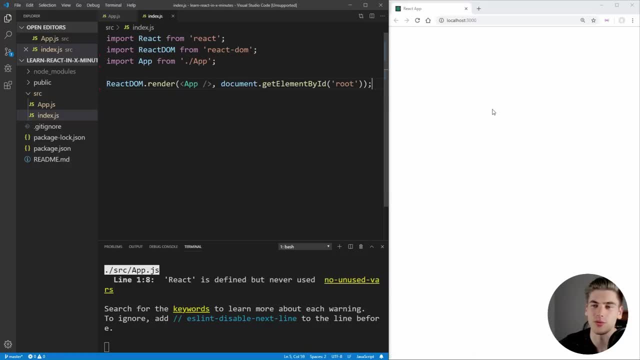 worker code, this css file or this service worker import here. we can also remove this service worker down here. now, if we save that, you can see we're back to our blank application and we just removed a bunch of the extra stuff that we're not going to be using in this application. and when you're starting with 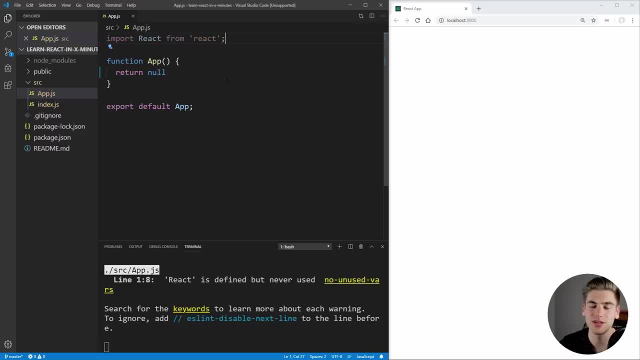 a react app. the first place you're going to start is your app component, because this is the root of your entire application and for our application, what we're going to be doing is building a really simple to-do list application. i know to-do lists are not the most interesting thing to build, but 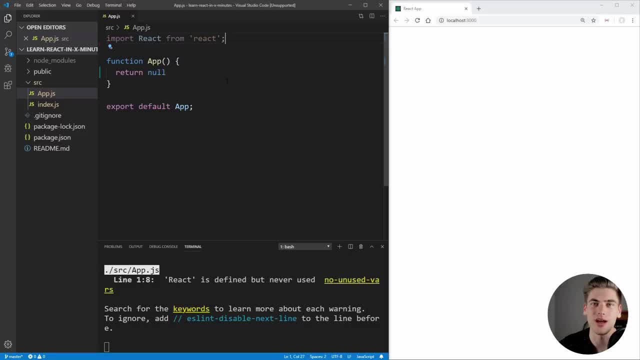 they are so good at showing all of the things that you need to learn with react in a really concise manner. so, to get started, the first thing that i want to do is actually write the html for our application, and we're going to start inside of our app component and return some html. 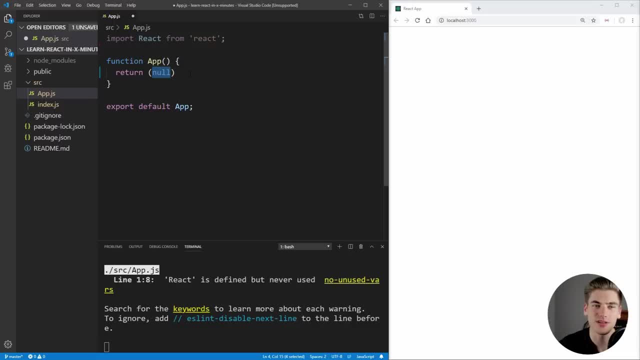 inside of here, and a trick you can do is to use parentheses in order to return everything inside of those parentheses and we then we can actually go on to a new line which allows us to just format our code a little bit nicer. so that's just a quick tip there for you, and the first thing we 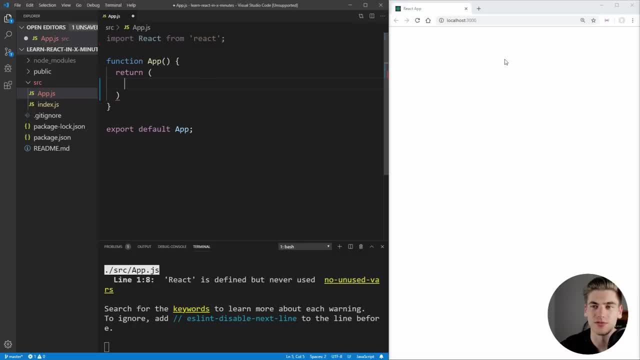 want to do is we want to return our to-do list. so our list of to-dos- and this is actually going to be be a separate component, So we're going to create a component called to do list And we're going to return that here as the first element inside of our application. And this isn't normal HTML, As 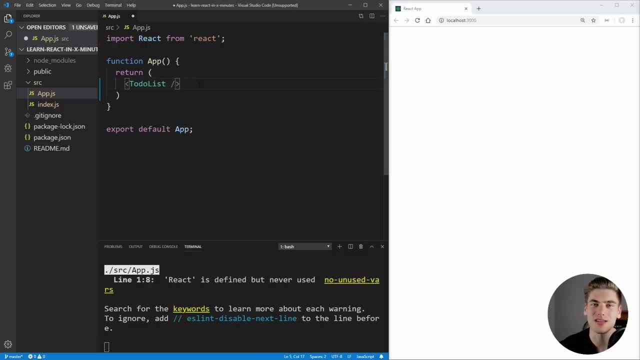 you can see this is not valid HTML, but it is JSX, which is kind of like reacts version of HTML, And it allows you to embed components inside of other components. You can see on our index: here we have our app component being embedded And inside of here we have a to do list component. 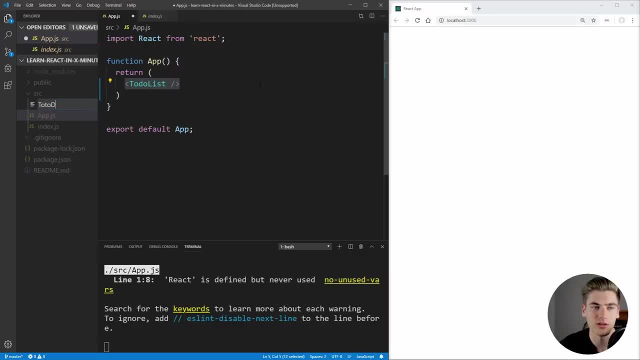 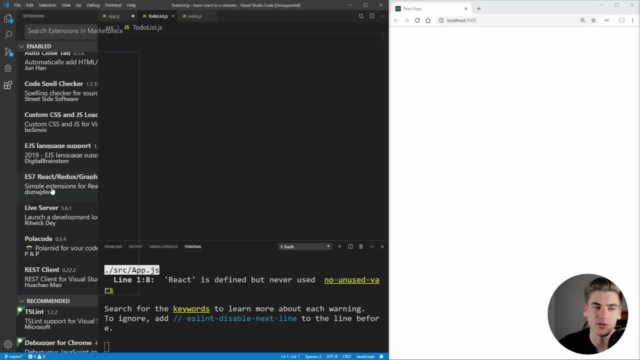 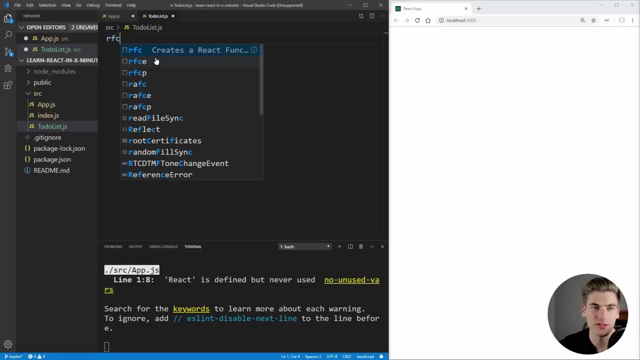 So we can just create that by saying new file, we can call it to do listjs, And I have a plugin installed on Visual Studio Code. If I scroll down here it's called ES7, React, Redux, GraphQL, Rack Native Snippets, And what this allows me to do is actually just type in RFC and hit enter. 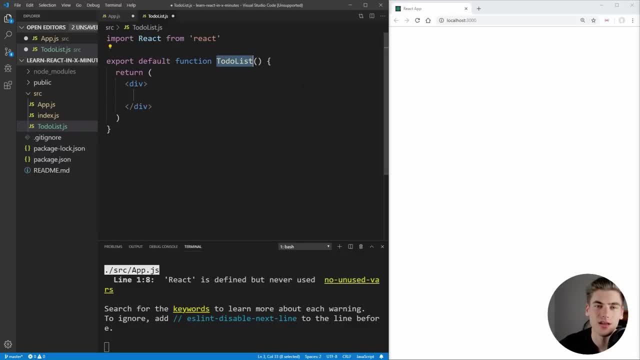 and it will create a function component for us inside of React And it will give it the name to do list, which is the name of our file. Now, instead of here, we can import that to do list component And we want to import it from dot slash to do list. So this is getting our component from inside. 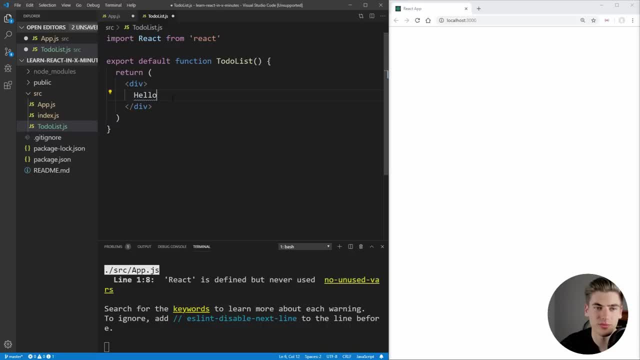 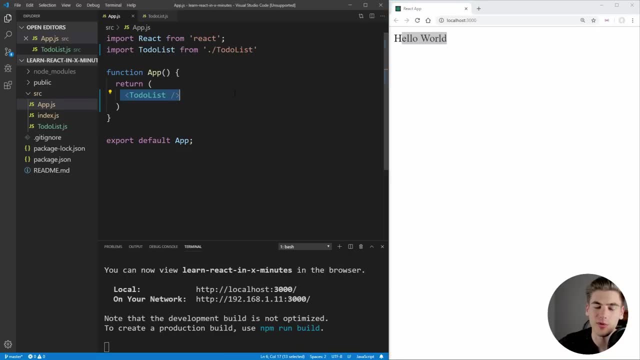 of here And we can just say Hello world, for example, inside of our return. And if we save that and we save our app over here, you see, Hello world is showing up because in our app we're rendering. 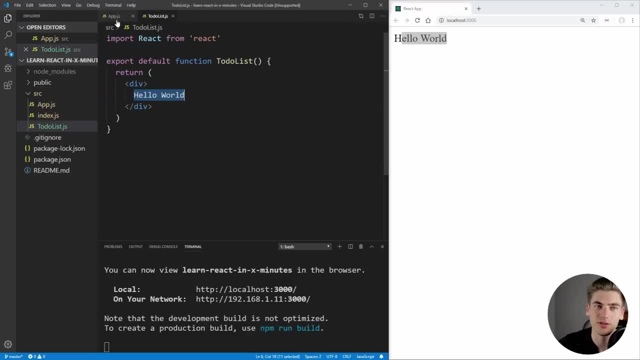 to do list, And in to do list we're rendering the text Hello world. So now, inside of our app, the next thing we want to do is put the input for adding a new to do, So we can just put an input. 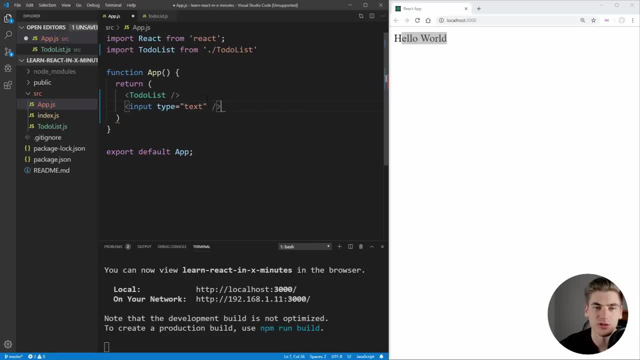 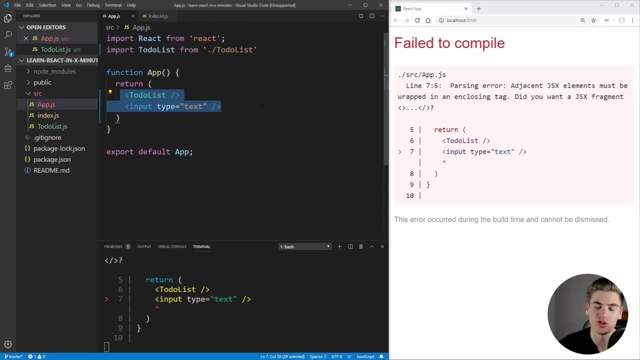 and we want to make it a type of text here And let's just close that off And if we save, we're immediately going to get an error, And that's because we can't put two HTML elements- or JSX elements in this case- next to each other. 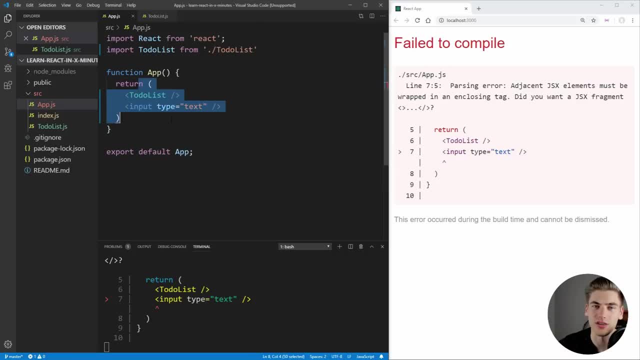 inside of a return, because this return can only return one thing. Any JavaScript function can only return one thing, And right now we're returning two things: a to do list and an input. So what we can do is wrap this inside of an empty element. This empty element is called a fragment And it 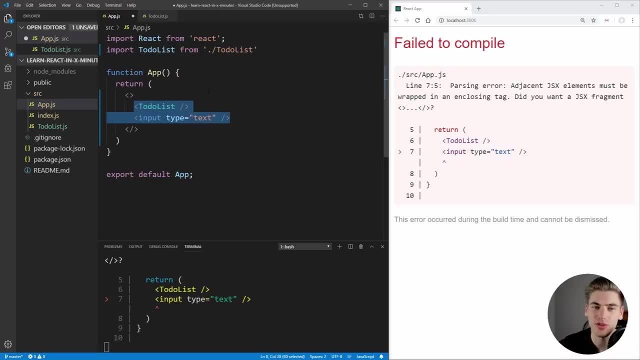 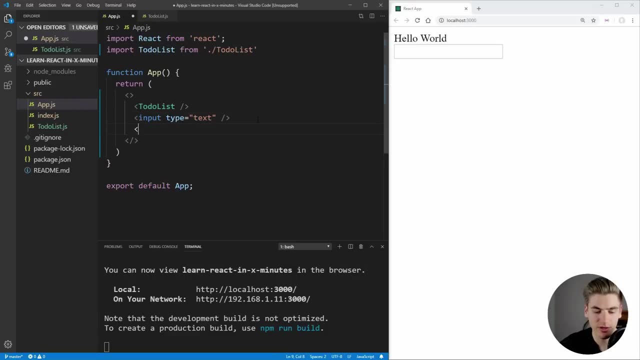 allows us to return one thing, which is this fragment, And we can also return one thing, and we can also return the other thing, which contains two things, which is actually what we want to return. Now we have that to do list text as well as this input here Next up, I just want to add: 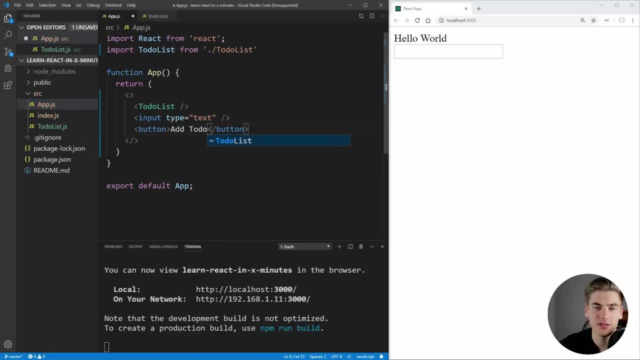 a couple buttons. This first button is going to be for adding our to do, and then we want a second button which is going to be for clearing our to do. So we'll just say clear, completed to do's. And then, lastly, after this, we're just going to put a div which says how many to do's we. 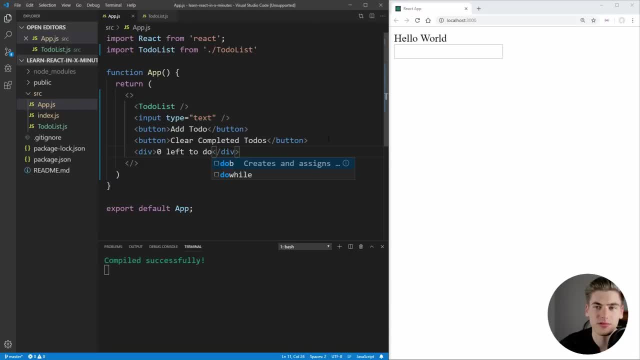 have left to do. we're just going to say zero left to do. Now, if we save that, you see we have our add to do button, our clear completed to do's and zero left to do, And let's just shrink down. 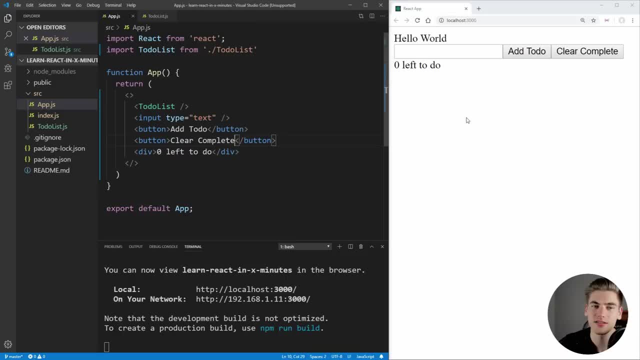 this name a little bit so we can get it to fit all in one line, just like that. And that's really all the HTML for our app component. All of the HTML for each one of our to do's is going to go inside of our to do list component. But before we can get started into that, first we need to set. 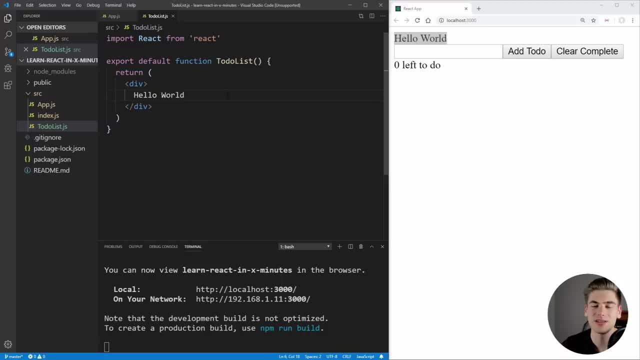 up the state for application. because the way react works is it manages state inside of your application And when that state changes it re renders things for us And we want to store all of our to do's inside of a state So we can actually render those to do's And every time we 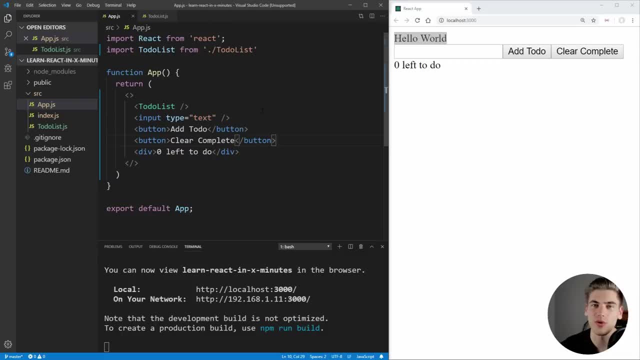 change it to do, added to do, deleted to do. it'll actually re render our entire component tree for us. So in order to use state in a function component, we need to use what's called the use state hook So we can import this from react like this inside these curly braces: 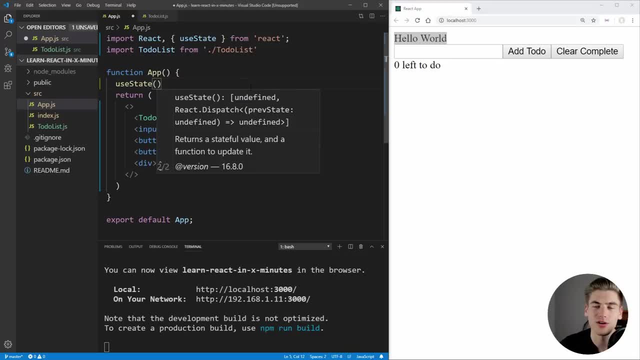 And now we can call the use state function And we want to pass it our default state For our to do's. the default is going to be an empty array. So the first time our app loads we're going to use an empty array of to do's, because obviously we have no to do's. And now 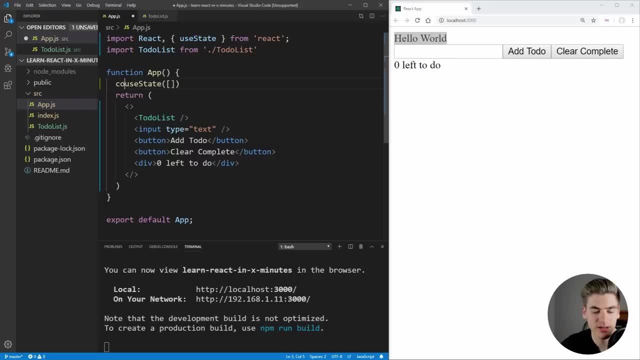 we need to set this to a variable here So we can say const. And the interesting thing about use state is it actually returns an array, So we can destructure that array and then set it equal to use state. And the first element is all of our to do's And the second element is going to be a. 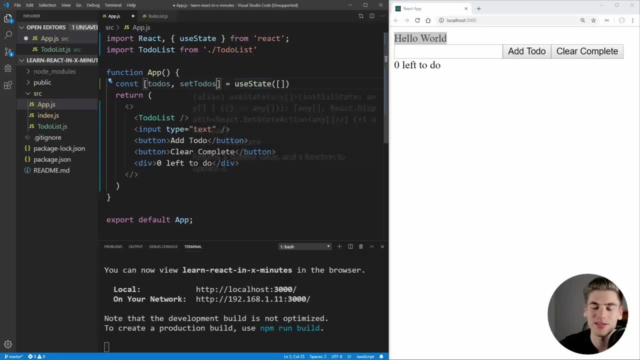 function that allows us to update our to do's, And this is a little bit confusing to look at. Essentially, this is just object destructuring, So if you don't know object destructuring, make sure you check out my video that I have done on object. 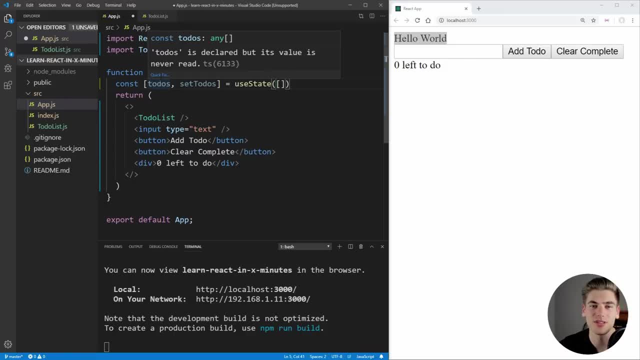 destructuring. It's linked in the cards and description below. But essentially this first variable here, to do's- is every single one of the to do's inside of our to do state, And the second variable is the function we call to update those to do's. To show you a little bit of, 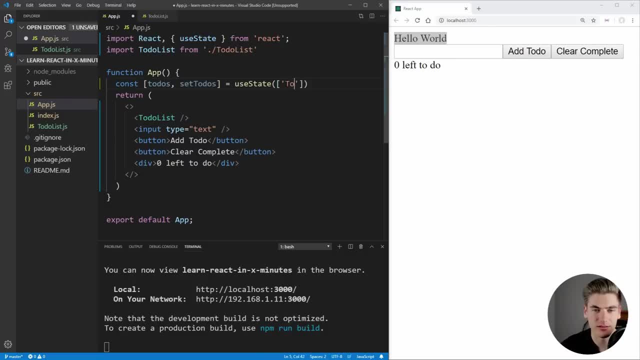 an example of what this would look like with actual data. let's just pass in some default data. we can just say to do one And we can have in here to do two as well. So now we have to do's by default inside of our application And we can pass these two are to do list by just saying to do's is going. 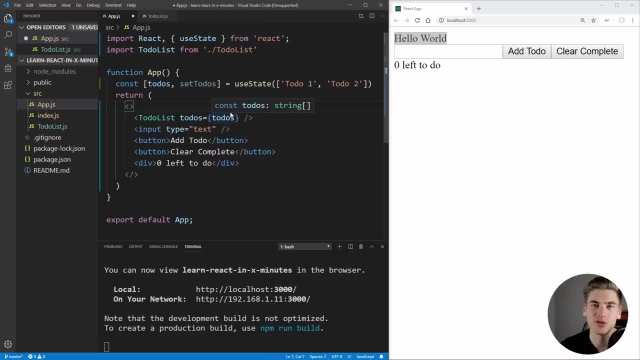 to be equal to do's, And this is what's called props. Essentially, all of our components, like app or like to do list, are going to have props that we can pass to them, And we pass them just like we pass attributes to an HTML element. So we're saying that we have a prop to do's. 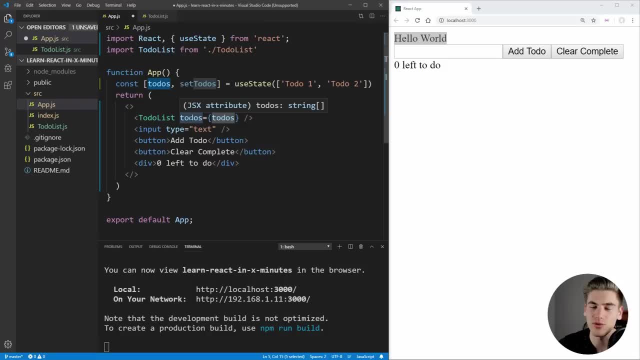 on our to do list And we want to pass the to do's variable to that prop to do's. we can have these as different names. this could be called to do list, for example, and it would be exactly the same. we would just have a to do list prop on our to do over here. So instead of 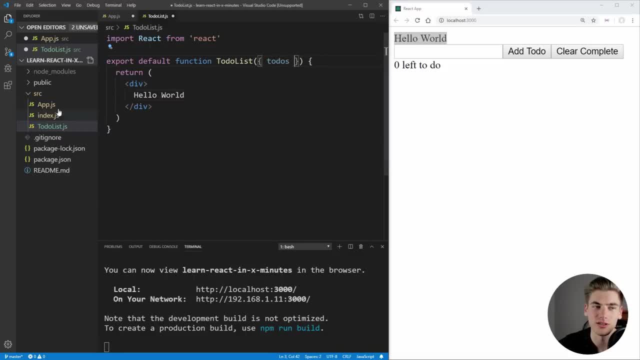 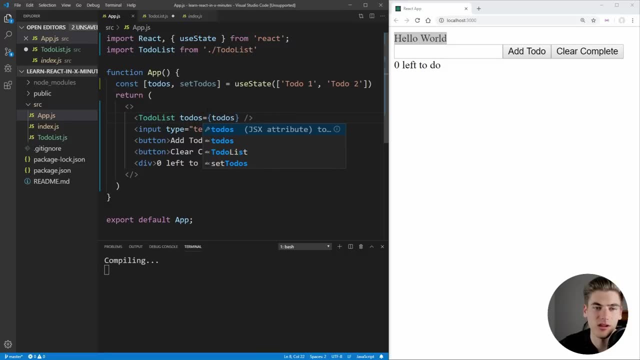 here this would say to do list. In our case we're just going to call it to do's because I think it's easier to work with. So let's make sure we change this also back to to do's And now inside of our to do list we can actually render out those to do's. So for now let's just say to. 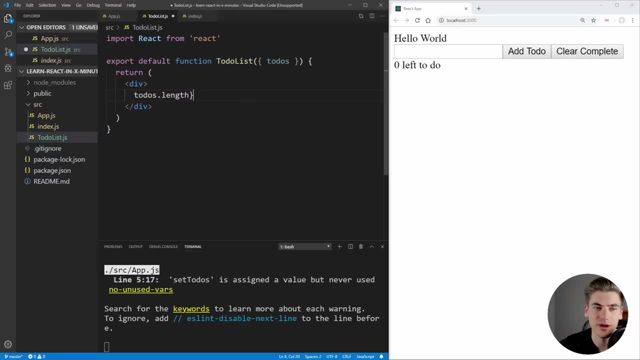 do's dot length And we need to put this inside of curly brackets here And that says that this is going to be JavaScript code. Now, if we save that, you can see it prints out two, because we have two to do's in this list, But obviously just printing out the number of to do's we have. 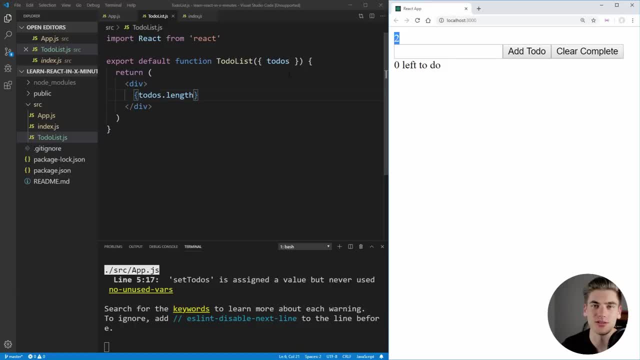 is not that useful. We actually want to print out each one of our to do's- And we can do that really easily inside of a loop- And what we want to do is actually map over our current array and return elements of our actual to do's, And we're going to do this with a to do component. 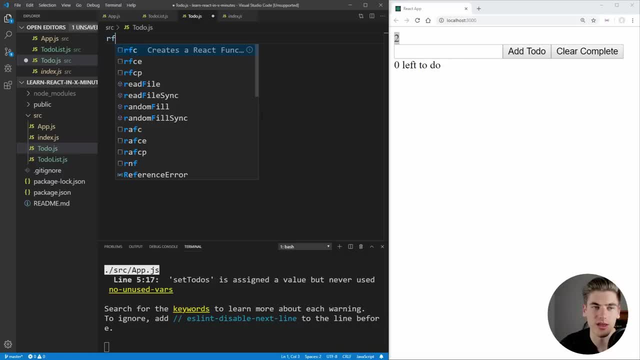 So let's create that to do component And of course we want to do that RFC trick in order to generate all the boilerplate code And inside of here we're just going to pass in a to do element, just like this. Now we can just save that, go back into our to do list And we want to import. 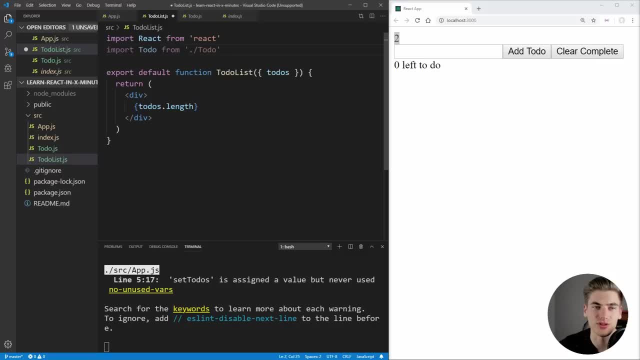 to do from dot slash to do just like that. Now we actually have our to do element inside of here to do component And what we can do is inside of an array we can actually loop over this So we can say: to do's dot map. 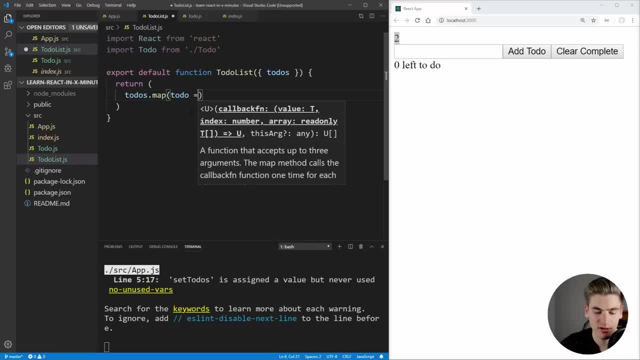 And we want to do is we want to map over all of our to do's. So, for each one of our to do's, we want to return a to do element, a to do component, and we want to pass it our to do, just like this, And: 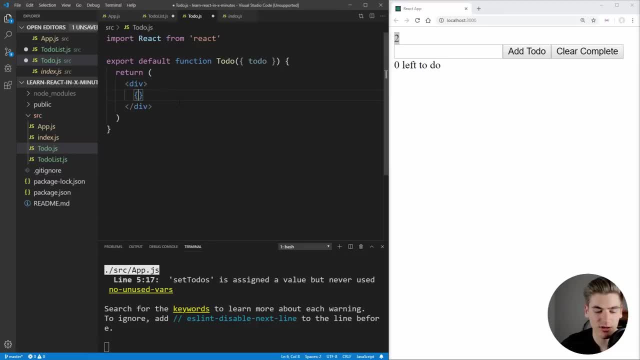 then inside of our to do, what we can do is we can just say: here we want to print out the to do, just like that. Let's save both of these And you can see immediately we have to do one being printed and to do to being printed. But there's actually a slight bug here If we inspect this. 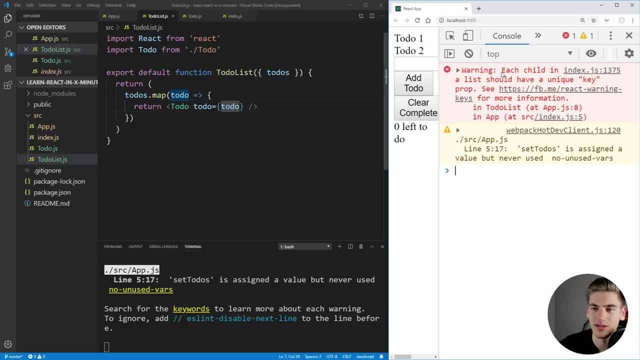 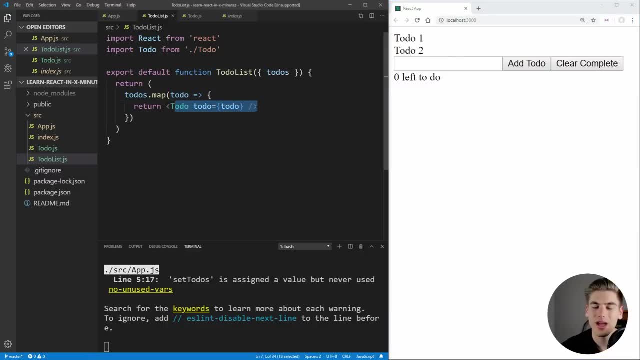 we're going to notice inside of our to do component- we have to do one- being printed And then inside of our console that we're actually getting an error. It says warning: each child in a list should have a unique key prop And what that's saying is that this list of to do's react. 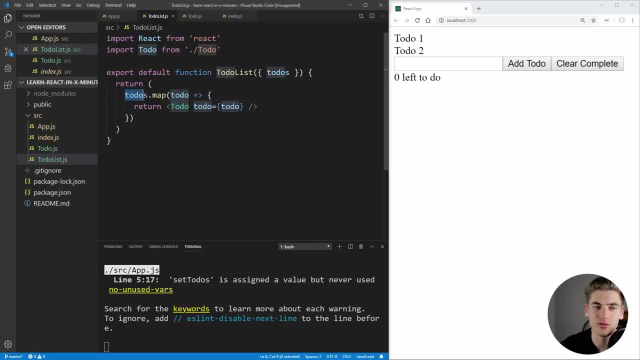 it doesn't know how to update these properly. Every time our to do's array changes, it's going to re render every single to do in that list, But we only want it to re render the ones that change. So what we can do is we can set a key here. In our case it has to be a unique element, So we can. 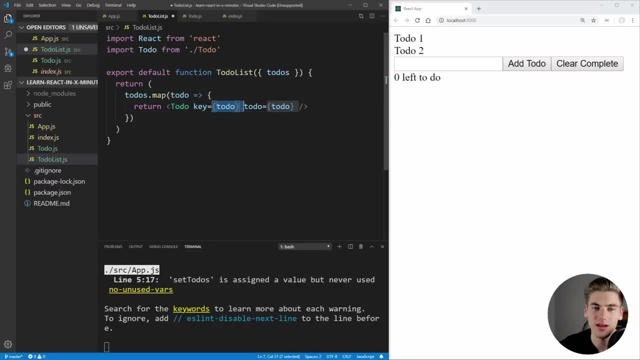 just set it to our to do name, which is right now unique. Anytime that you want to do that, you can have a key. you just need to make sure that it's unique for the array that you're actually using it with. In our case, the name is going to be unique. Now, if we save that and go over and inspect, we 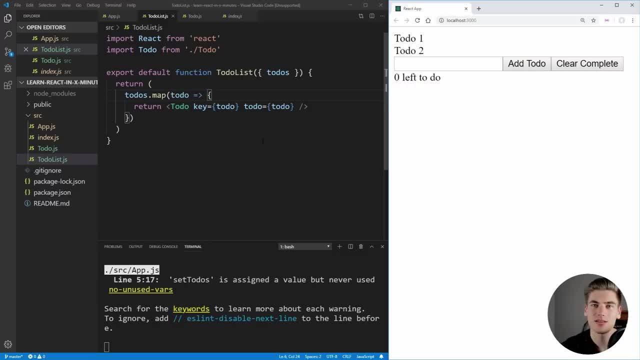 no longer have that error, as you can see. So that's perfect And essentially what this key does is it allows react to only re render or change the components that actually change inside of our array, Instead of re rendering all of them every single time. It's really there for. 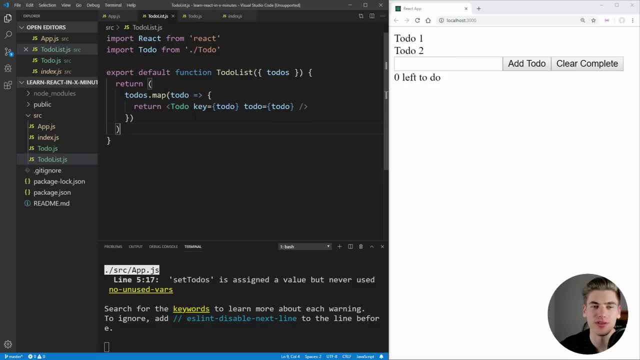 efficiency purposes. Now, obviously, we can't just store the name of our to do. we actually need to have an object of whether or not it's complete. we need to have an ID as well as a name. So back inside of our app, let's actually change this array to be an object. we're going to have an ID of one. 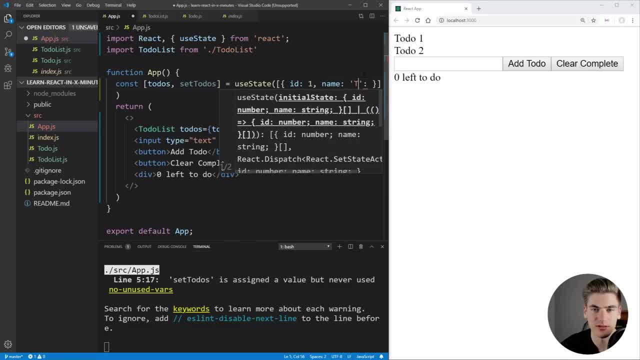 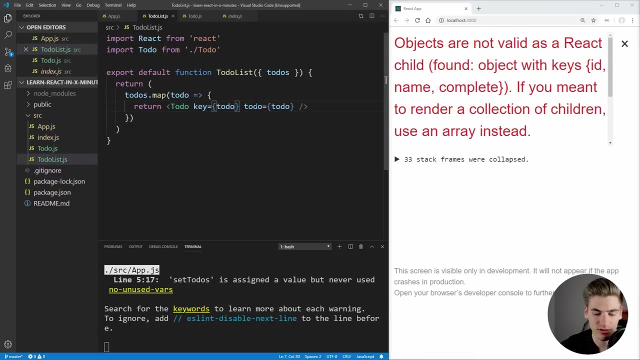 we're going to have a name which is just going to say to do one, And then, lastly, we're just going to have a property called complete, which we'll just set here to false for now. So now we have a to do with an ID, a name and a complete flag, And then, instead of our to do list, we can just use to. 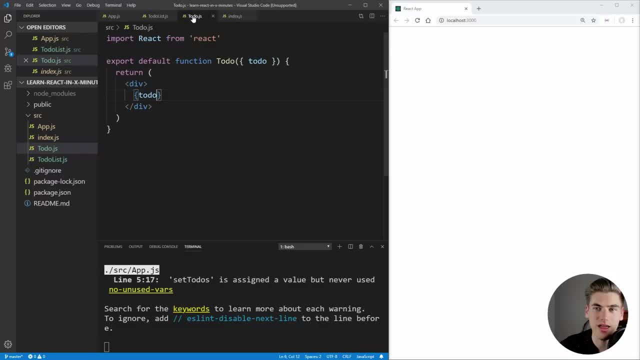 do that ID here And then inside of our to do. we want to just print the name So we can say: to do dot name. Now you can see, to do one is showing up, perfectly fine. But obviously we don't want to just have the name being. 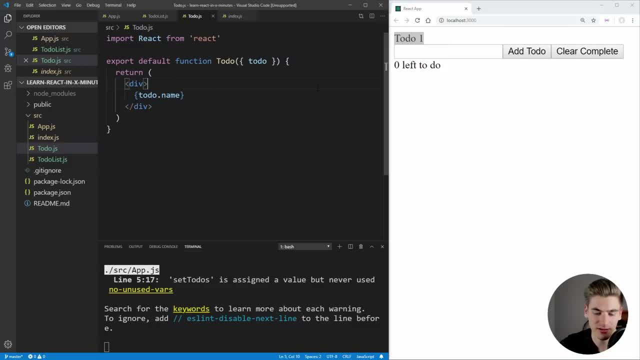 printed out. we actually want to checkbox to check whether it's complete or not. So let's set up all of our code for doing this. First we're going to have a label, And inside of this label we're going to put the two dot name, just like this. make sure I get rid of that. And then inside of here we also. 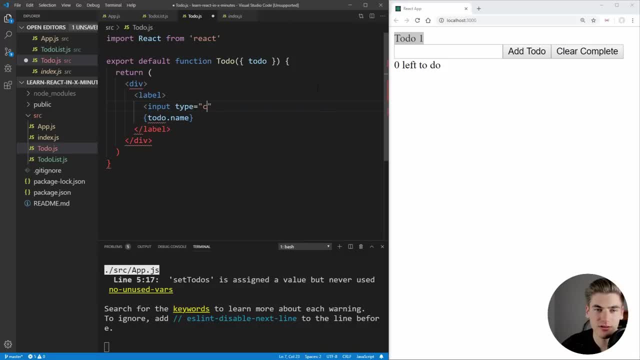 need our input type of checkbox, just like that, And we also want to set in here a checked property, essentially the value, and we want to set that to, to do dot complete. And now, as you can see, we have our to do with our. 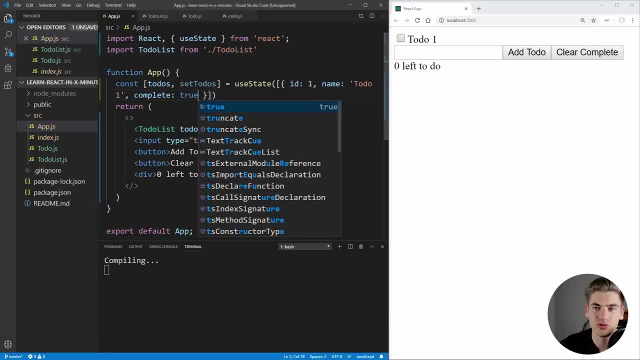 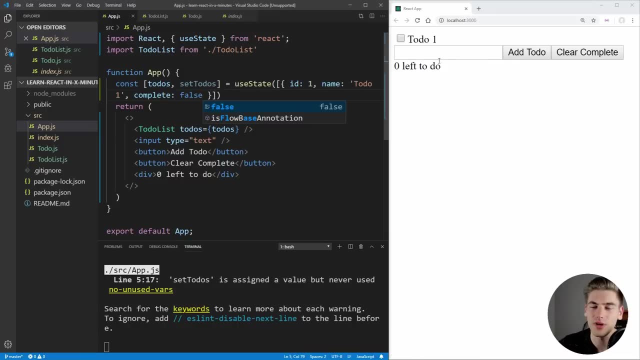 checkbox over here And if we come over and change our complete value to true, you can see it's going to check our checkbox for us, And if we have it as false, obviously it's not going to be checked. Now what we need to do is actually set up events so that we can actually add to dues. So let's remove. 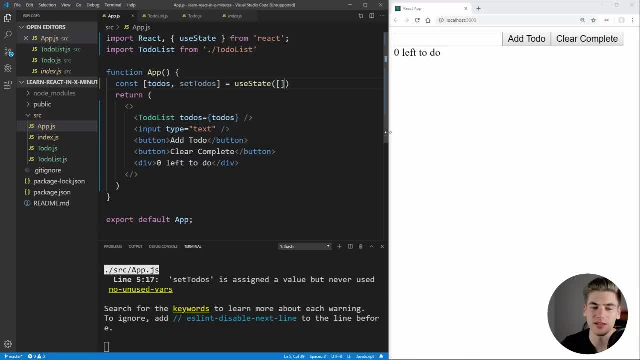 this default to do for now and just have an empty array because by default we're not going to have any to dues at all in our application when it starts up. But we do want to add to dues whenever we add this to do with. 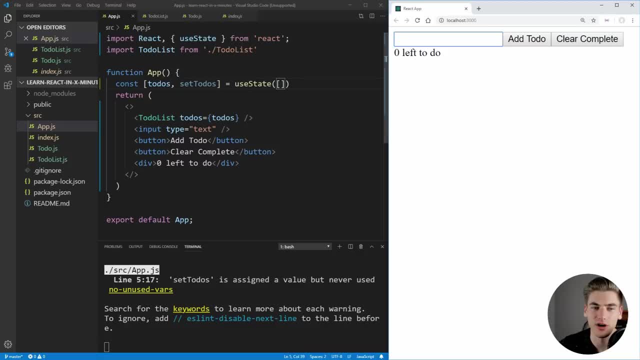 the add to do button. So we need to set up an on click listener on our add to do button. So we can just say on click. And we want to set this equal to a function. In our case, we're going to call a function. 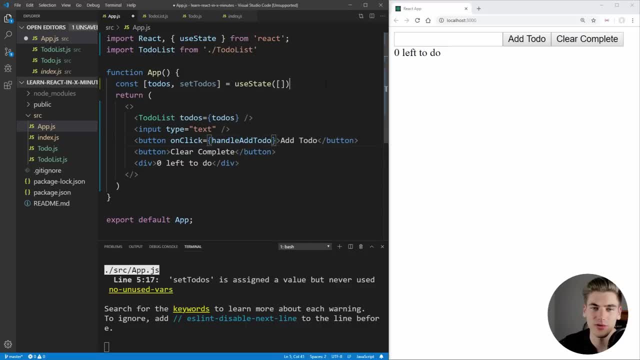 which is just called handle add to do, And let's create that function up here. we can just say function handle to do, And it's going to take that event property And inside of this function what we need to do is 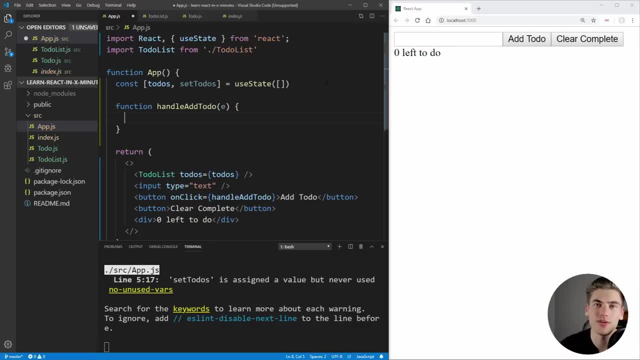 we need to set our to dues to one more. to do So, we need to take our previous to dues, add our new to do and then set our to dues to that to do list. But you'll notice one problem immediately: we don't. 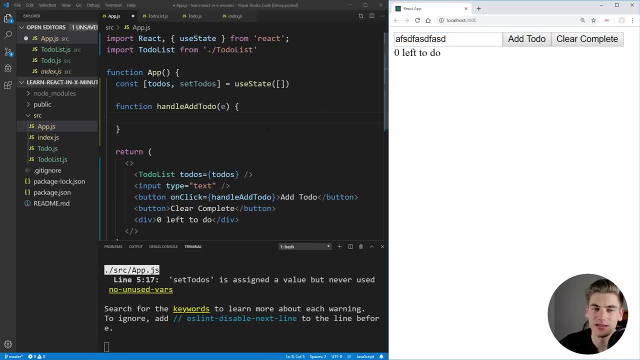 have access to the name inside of this field. we can type this in click Add to do. it's going to call this function, but we need access to this name And this is where what's called the user ref hook comes in handy. So we can say use ref And the user ref hooked allows us to. 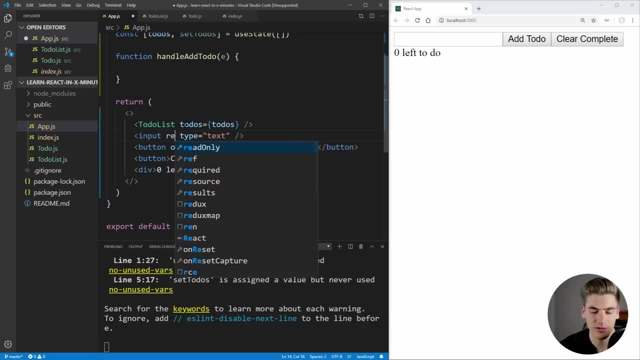 reference elements inside of our HTML, in our case the input. So we can say: ref here is going to be equal to a variable. we're just going to call this to do name ref And then we can create this variable up here by just saying const to do name ref is equal to use ref. Now we're going to 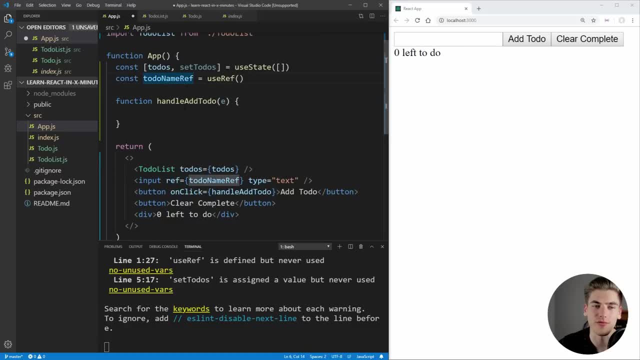 have access to this input element inside this to do name ref variable. And to access it we just say: to do name ref, dot current, which is going to be whatever element we are currently referencing, in our case this input. So we can say dot current, dot value And this is going to be the value of our input. So we can just 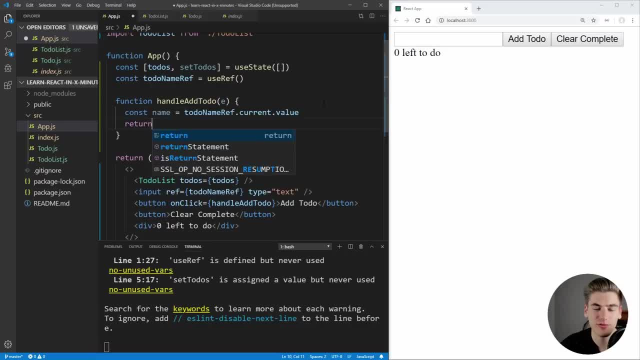 say that the name is going to be equal to this, And then we of course want to return if our name is equal to an empty string. Essentially, if they don't type in a name, we just want to return so we don't add an empty to do, And then afterwards. for now, let's just log out that name to make sure. 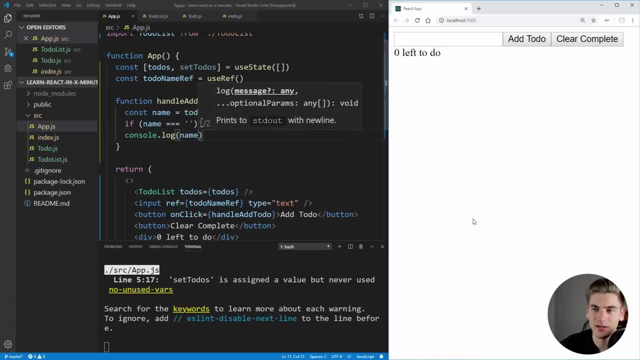 that this is working just like that. So now let's inspect this page, go over to our console And if we type in a name, for example, we can just say hi, click Add to do. you can see it prints out high. If we 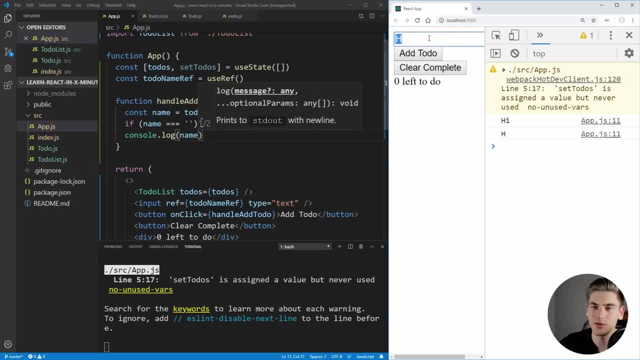 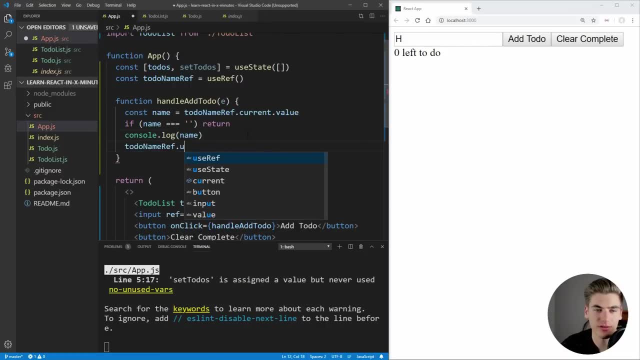 type in just H, hit Add to do. it's going to print out H, So we have access to whatever is inside of this variable here, inside of our input. One other thing that we probably want to do is we want to take our to do name dot, ref, dot, current, And we want to set the value here equal to null. That 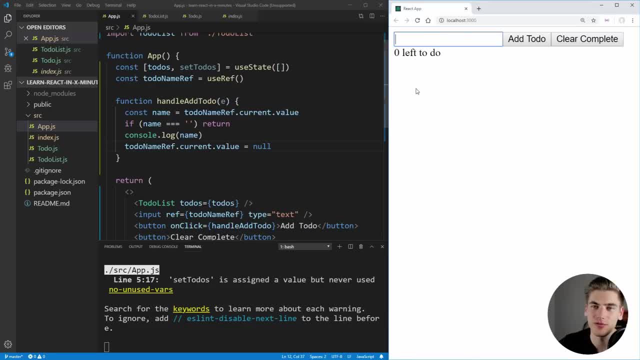 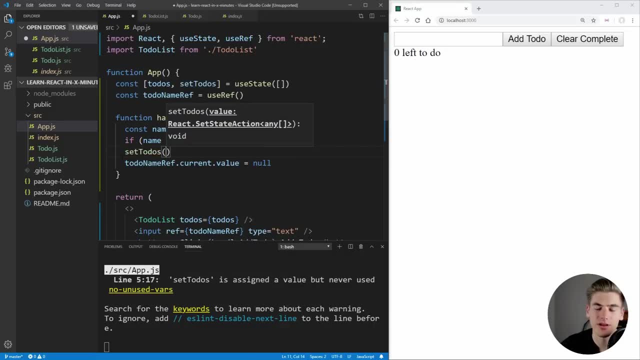 way, if we type in something and hit Add to do, it's going to clear out our input. for us, It's just a nice quality of life change. Now, the real change that we need to make is actually setting our to do's. And the way set to do's works is you have two different ways you can set them. you can 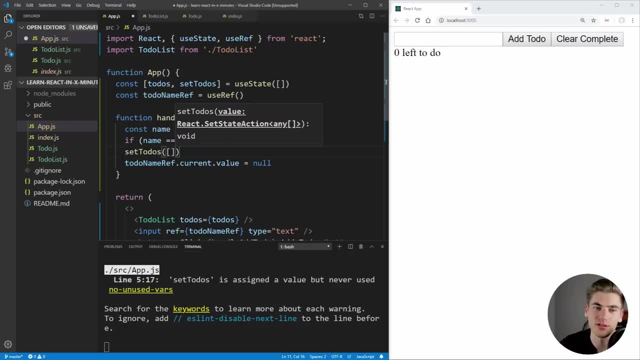 just pass it. a value, for example, empty array, would clear all of our to do's, Or you can use the previous value. In our case, our previous to do's is a function call, So it's a function that is going to give us the previous to do's, which allows us to change that. So we could say that now. 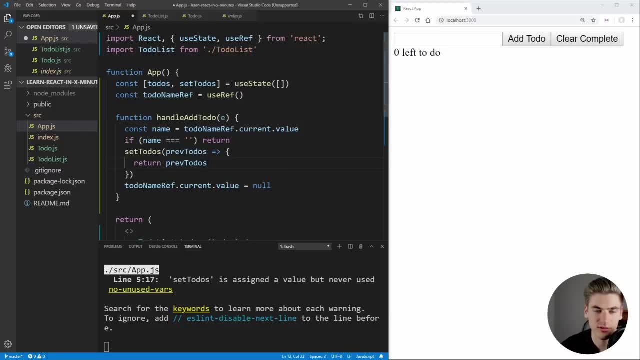 our new to do's is going to be equal to previous to do's And we want to spread this over our array, And then we want to add a new to do to that list. So let's just, for our case, give it an ID of one, a name, which is going to be equal to our name. 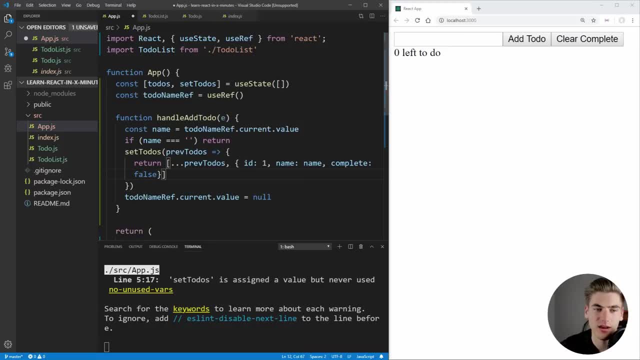 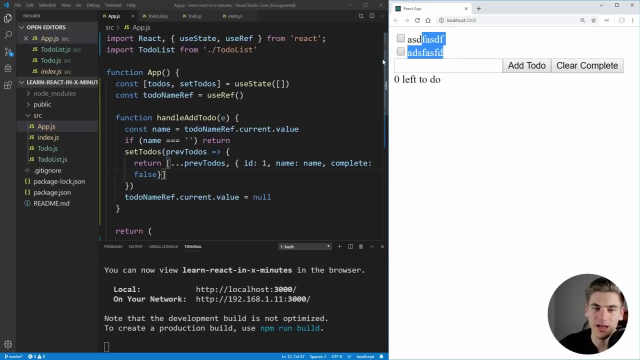 variable and a complete of false. Now what we can do is, when we save this, we type something and hit Add to do. you see it's going to add that to do, But the problem is we're always adding with an ID of one And if we inspect our page we should see that we have an error inside. 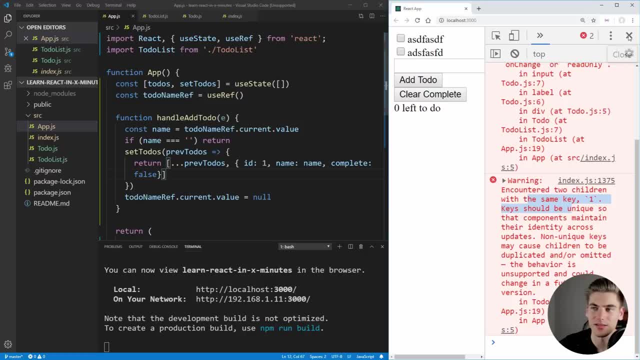 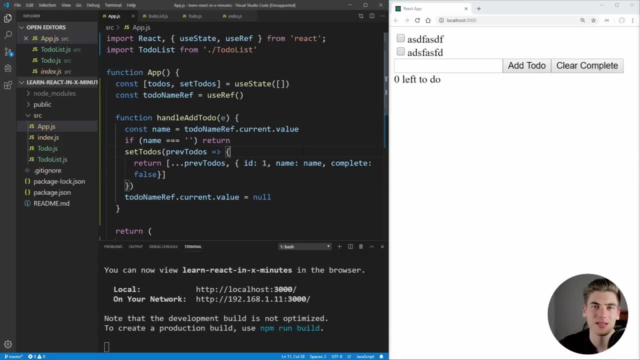 of our console, which is saying that we have two keys with the exact same ID. So what we need to do is actually download a library that's going to allow us to completely create random IDs, And the best library for this is called the UUID. So we can just say: NPM I UUID, just like that it's going. 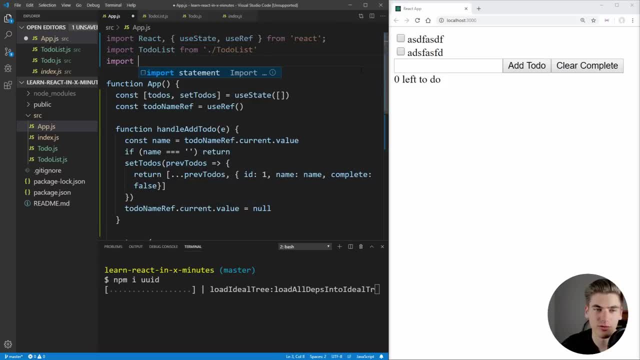 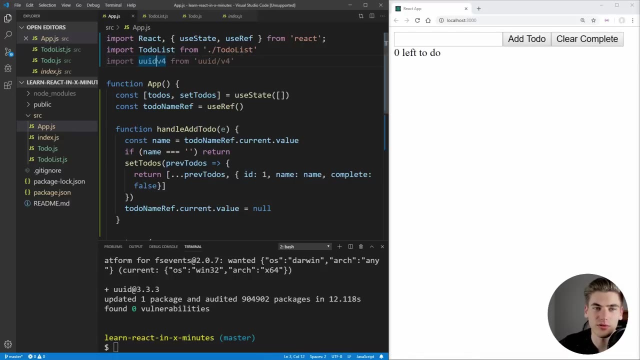 to download the library for us And we can actually import the UUID inside of our application. So we can say: UUID v four from, and we want to import that from UUID slash v four, just like that. This is going to give us access to UUID v four, which is just a function that generates a random ID. So 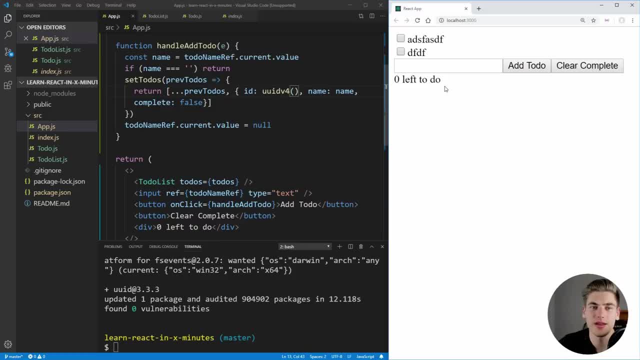 we save that, create some to dues. we're no longer going to get that error of having duplicate keys because our IDs are now completely unique. But you will notice a problem Every time we refresh our page. we no longer have our to dues being shown up. they're not being persisted across page reload. 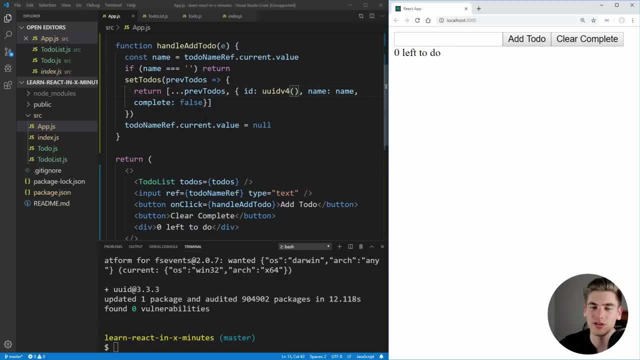 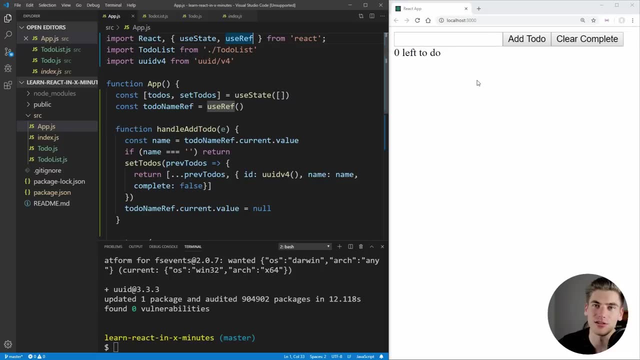 And this is something that's very easy to fix with react, we want to store these inside of local storage And the easiest way to do things which are a side effect. So, for example, every time we added to do we want to save it, we can use what's called the local storage, And this is what we're. 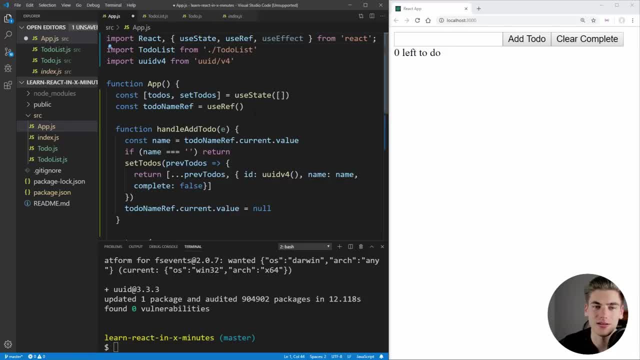 going to call use effect, which is just another hook inside of react, And this is just a function which is going to take as its first parameter another function And this is the function that we want to do things. So every single time something changes. we want to call this very. 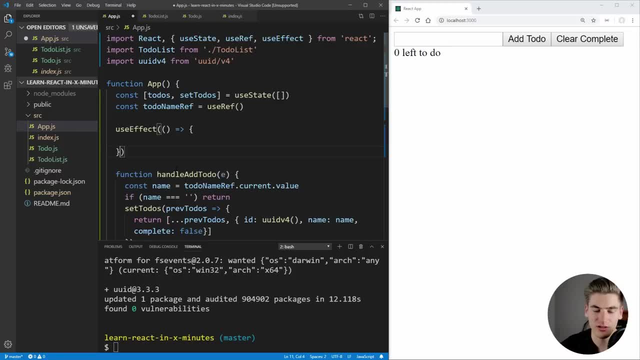 first function And the way we determine when to call that function is: we pass an array of properties here And this array is going to be all of our dependencies. So anytime anything in this array changes, we want to run this use effect function. So in our case, 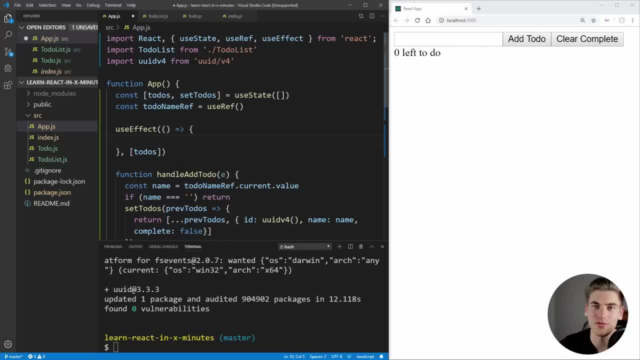 anytime our array of to dues changes. we want to save our to dues and saving them is really easy. we're just going to save them to stock local storage. So we can say local storage dot set item. we need to give this item a key here. So let's create a variable for that. we're going to call it. 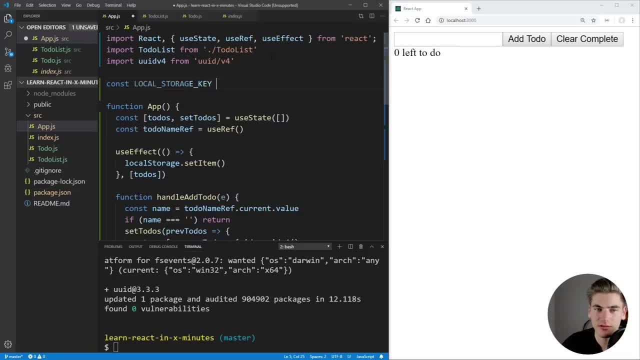 local storage key And we're just going to set that to deduce, to do app dot to dues, just like that. You can call this key whatever you want, it really doesn't matter. So we pass it, first, the key, and then we want to save our to dues, And then we're going to save our to dues And then we want. 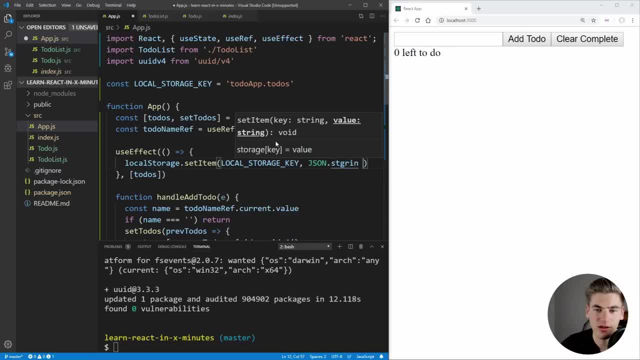 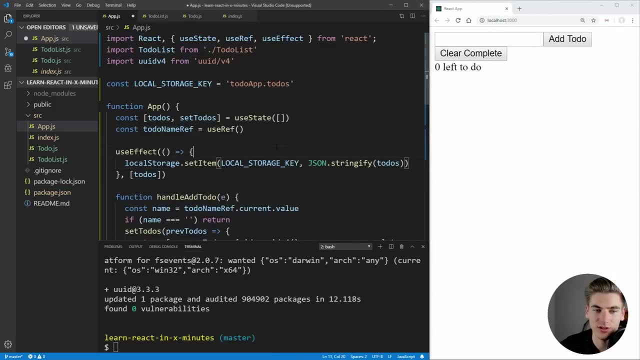 to make sure we pass it a string. So we're going to stringify whoops, stringify our to dues. So this is just a JSON string of our to do application. There we go. So now we added to do, add another to do. it's actually saving these to our local storage, But of course, when we refresh they're. 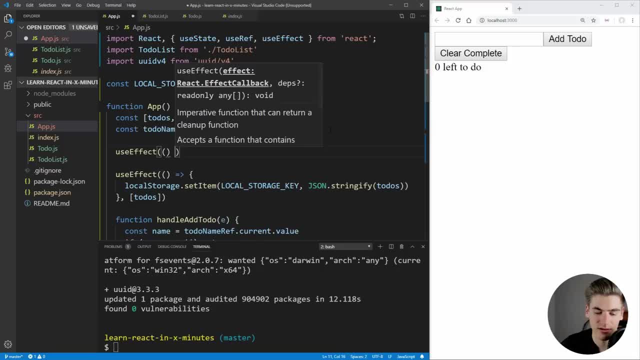 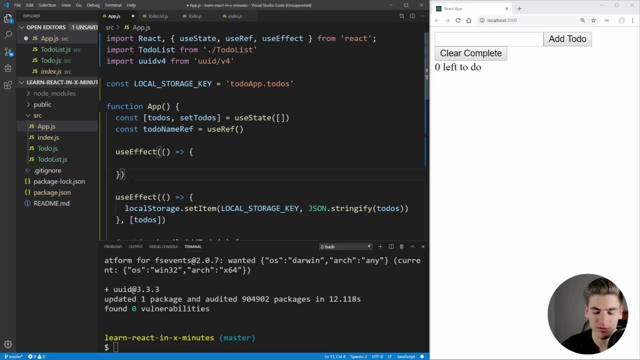 not showing up And that's because we need to use another effect, And this effect we're going to call to load our to dues And we only want to call this once, right, when our component loads. So if we pass an empty array of dependencies, it'll call this function once And since the empty array 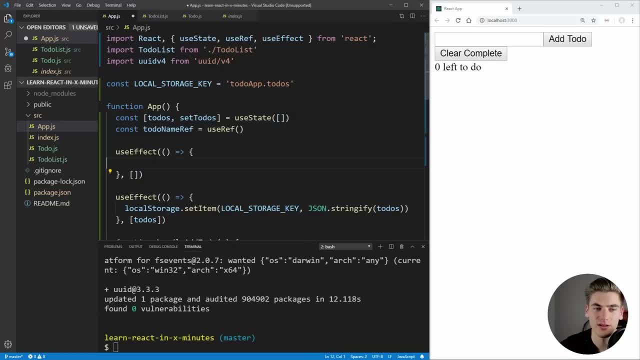 never changes, it'll never recall this use effect. And this use effect we want to set our to dues to what we get back from our stored to dues So we can say const stored to dues is going to be equal to local storage. dot get item of that local storage key And we want to make sure that we get that. 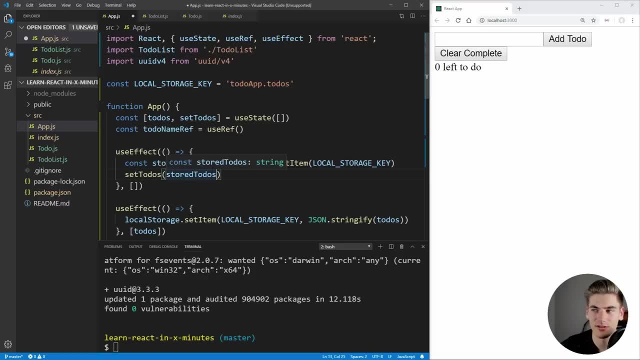 item stored into our stored to dues And then we want to set our to dues to that stored to dues only if we actually have stored to dues. So if we have stored to dues, then set our to dues to those stored to dues. Now, if I save that, you'll see we're getting an error And that's because this: 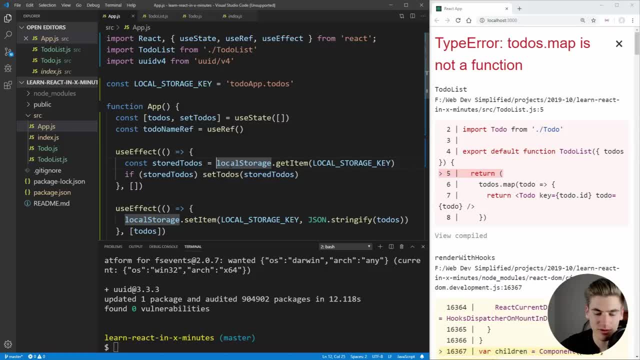 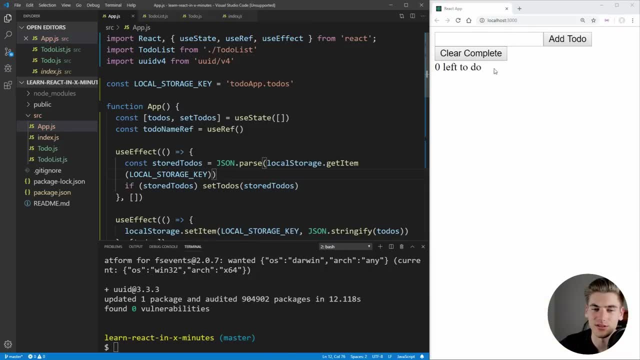 is a string. we need to parse this using JSON. So we can just say JSON dot, parse of that string. this will convert it to an array And now, if we save that, you can see that this is working properly. Now let's add some to dues. we'll say FFF, AAA, And if we refresh those to dues are: 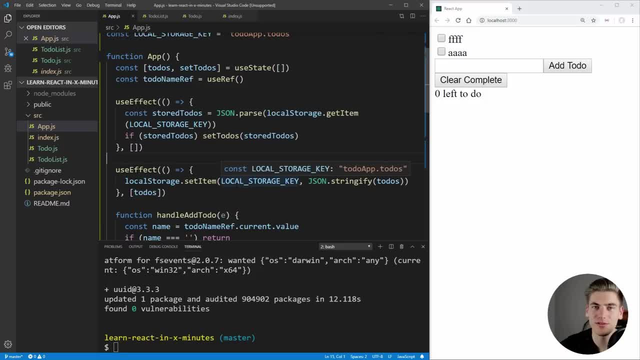 storing and getting our to dues is working properly. So now we have saving built into our application and only just a few lines of code, which is the real power of the use effect inside of react. Now this is all great, But right now we have no way to toggle our to dues, Even if we 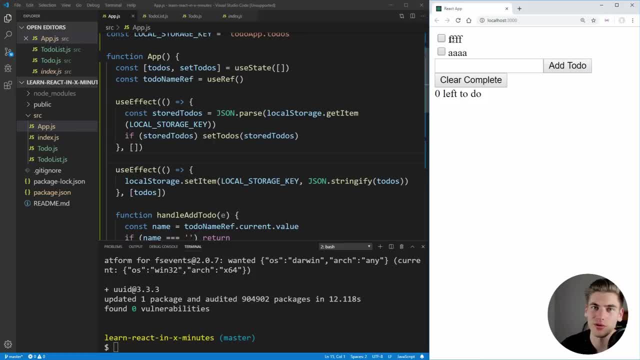 click on this checkbox, it's not actually going to check our to do. for us, we need to write some react code in order to store the change of our to do from being not complete to complete, or vice versa. So let's write a function to do that. 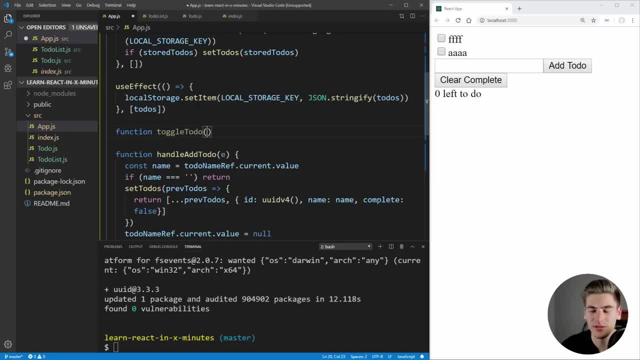 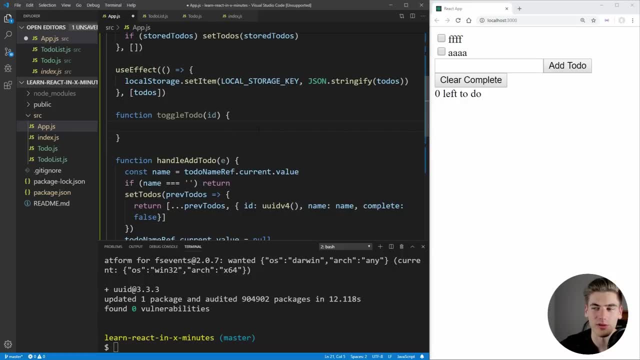 Here, create a function called toggle to do, And this is going to take just an ID of the to do that we want to toggle, And then what we want to do is we want to toggle the to do from our list. So the first thing we want to do is get a new list of to dues. we're just going to call this new to dues. 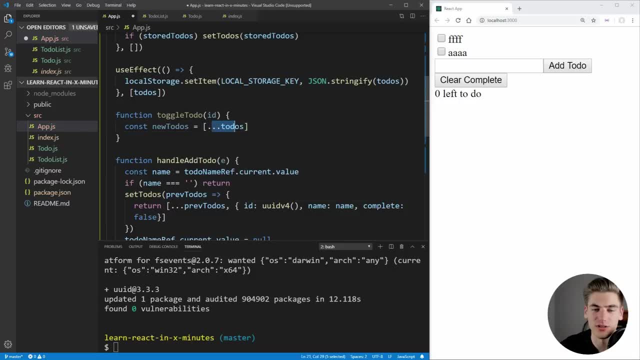 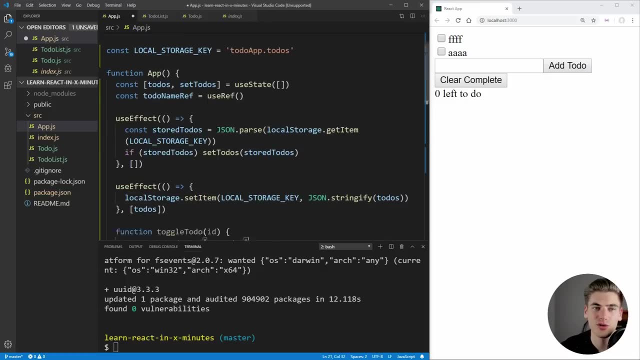 And it's just going to be equal to a copy of our current to dues list. This is just so we don't change our current to do list And we always want to make sure we create a copy. In react. you should never directly modify a state variable. you should always create a. 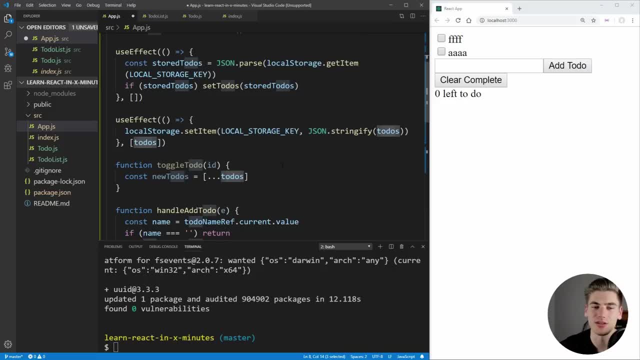 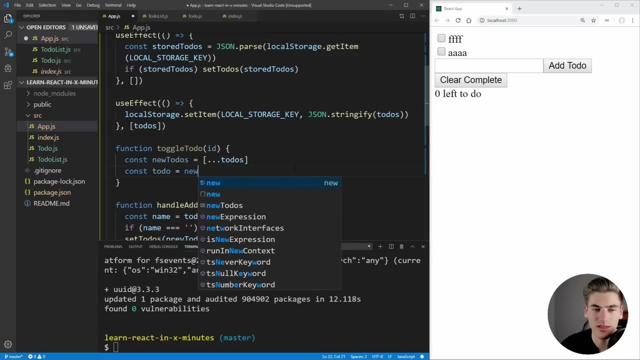 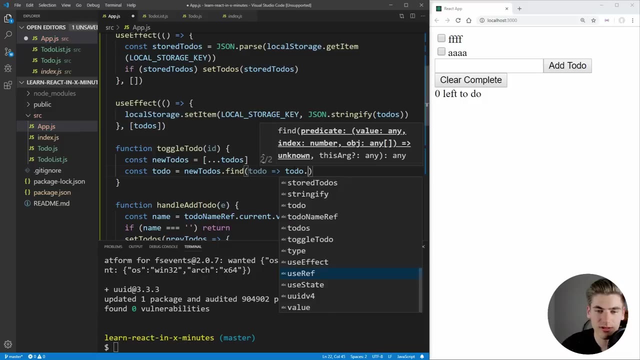 copy before modifying it and then use that copy to set the new state. So we've created our copy. Now we want to get the to do that are actually trying to modify So we can get that from our new to dues by just finding a to do that has the to do dot ID, which is equal to the ID that we 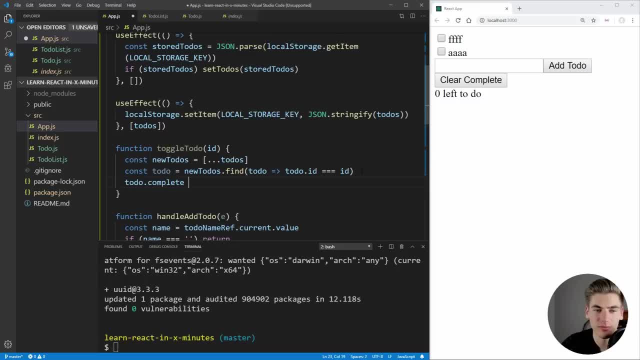 passed into toggle to do, then we can just say: to do dot complete is going to be equal to the opposite of to do dot complete. So we can just negate that here And then we can just say: set our to dues to our new to dues. This is essentially going to allow us to toggle or to 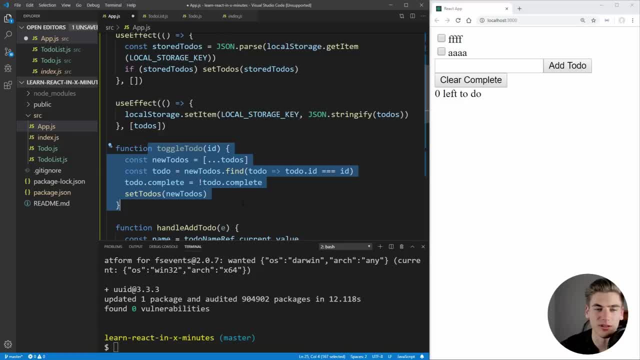 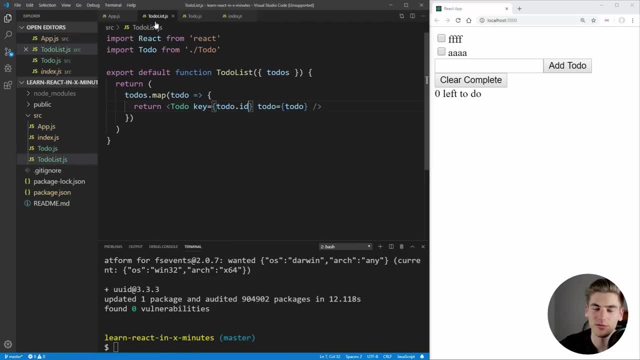 do from complete to incomplete or from incomplete to complete. But we don't have any way we can use that function Because, as you remember, our to dues are stored inside this to do component, which is referenced inside of our to do list, which is referenced inside of our app. So we 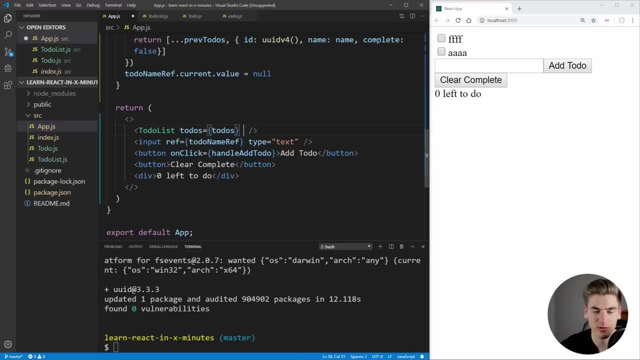 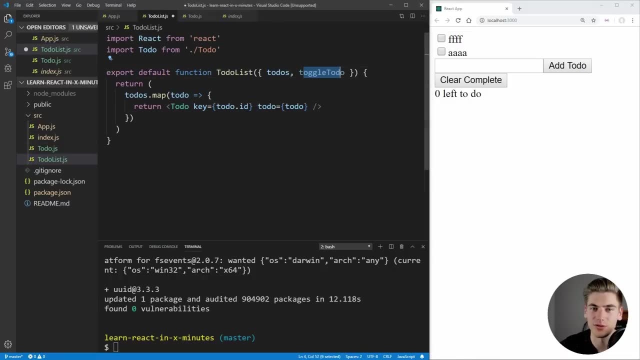 need to pass this function down into our to do list So we can just say: to do, toggle to do is going to be equal to toggle to do. then instead of our list we can import that toggle to do prop and pass it down to individual to dues, just like this. So now we're passing both. 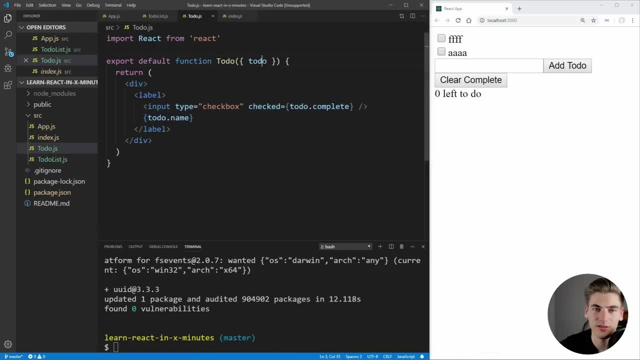 the to do and the toggle to do function And then finally, inside of our to do, we have that toggle to do function And on our input, we can come in here And we want to say, on change, we want to call a function And this function is not going to be our toggle to do, because we need to make sure. 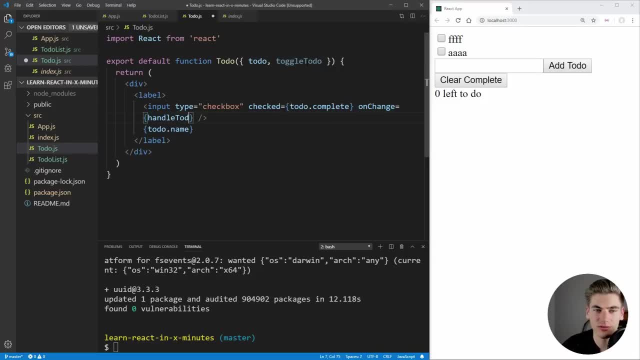 we pass an ID. So we're just going to say we're going to call this handle to do click And then we're going to create that function Which is handled to do click, And inside of this function all we need to do is we need to call. 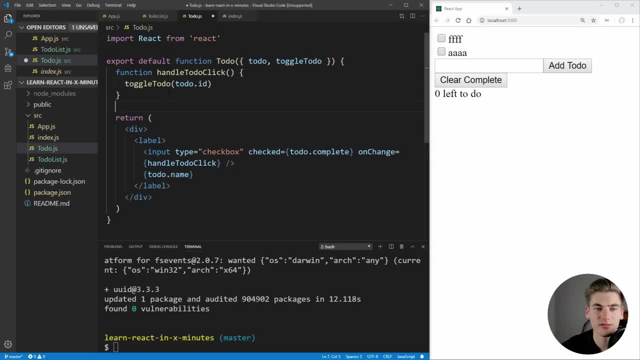 toggle to do and we want to pass it our to doid. Now, if we save that and we just click the check, you can see it's actually checking our box for us, Same thing with our A, And if we refresh, you see it storing that complete status inside of our to dues, inside of local storage And the way 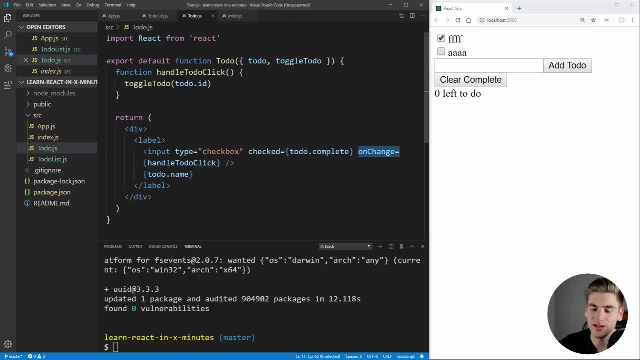 that this is working. it's a little bit confusing is what's happening is, every time we click is calling this on change, which is calling our toggle to do function, And then we're going to toggle to do function with the idea of the to do we're inside of. that in turn gets passed up. 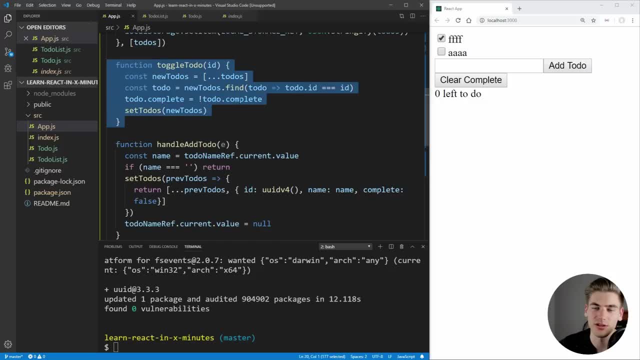 through to do list into our app, which calls this toggle to do function here, which resets our to do list variable to the new list of to dues with the to do checked that we clicked on. Now that we actually know how to toggle and untoggle our to dues, Let's make this text down here, actually. 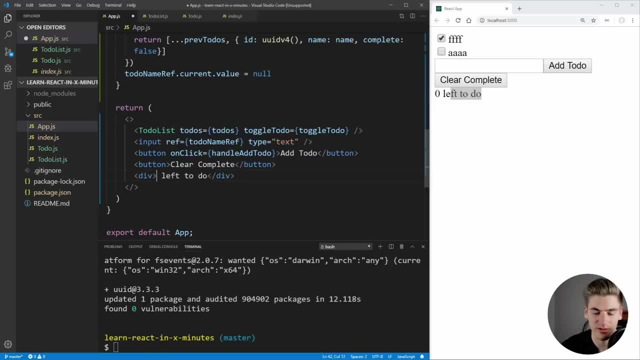 tell us how many to dues are unchecked. And this is fairly straightforward to do. we can just say to dues dot filter, And we want to filter all of the ones that are not checked. So we can say: to do which is not complete, just like this, And we just want to get the length of 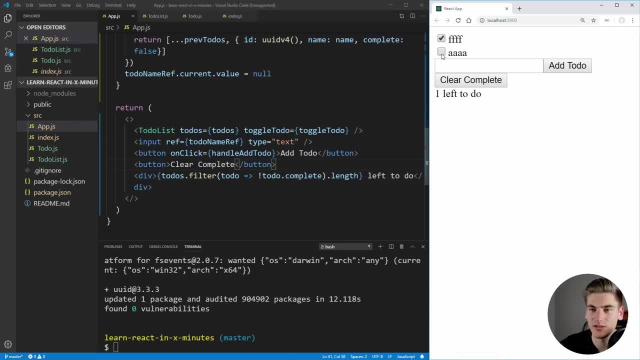 the not complete to dues. Now if we say that you can see we have one to do left, we check this. it goes down to zero. we uncheck both of them. it says two left to do and so on. And if we add, 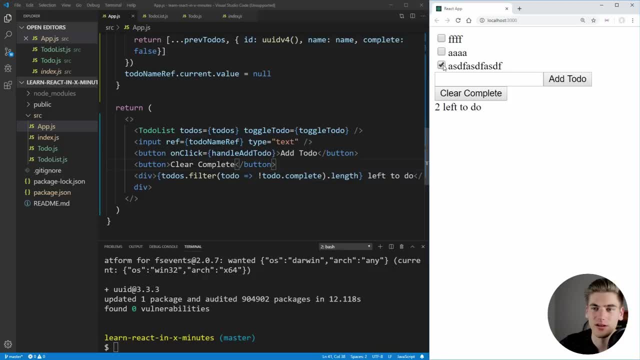 a new to do. it's going to go up to three, which is great. Now let's set up the click event listener for our clear complete. we can just come in on click. we want to handle clear to dues And we can.